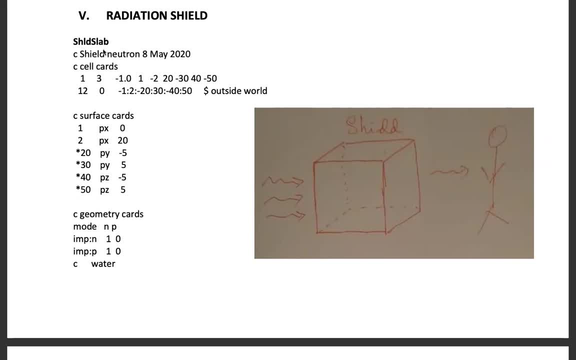 I have the title card that is a slab shield and this. I did the simulation on 8th of May 2020 and these are the cell parts. Now, again, I've got like Godiva. I had a sphere. now I've got a cube. A cube has six surfaces, so I need to have six. 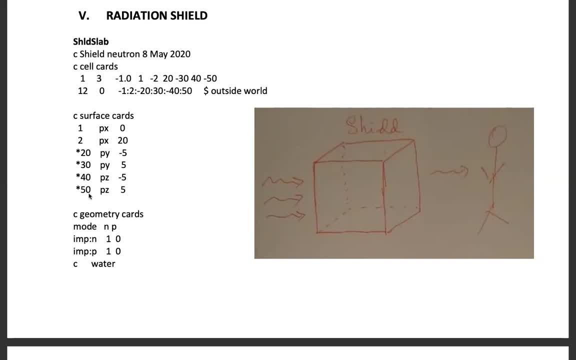 surfaces over here: one, two, three, four, five, six. Now, the first two surfaces are normal to the x-axis, so that x equals to zero and x equals to 20 centimeters. Surface number 20 and 30 are normal to the y-axis, minus 5 centimeter and plus. 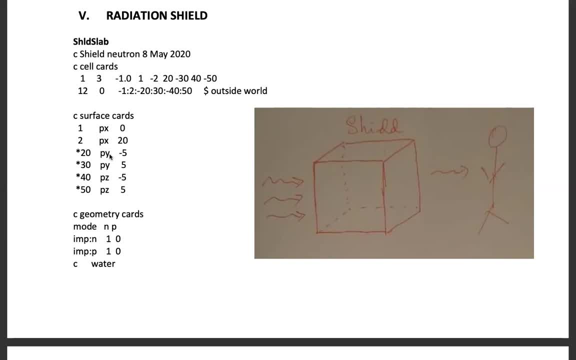 1 centimeter, which means that their of thickness, 10 centimeters On the y-axis. on the z-axis again, surfaces 40 and 50 have a thickness of 10 centimeters between minus 5 and plus 5.. So the 10 centimeters are actually minus five. 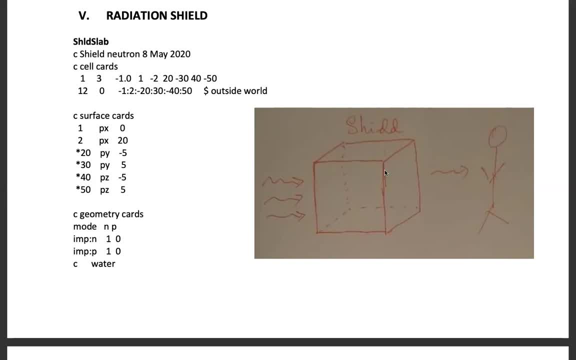 So let's say that this is the x-axis, and that's the y-axis, and that's the z-axis. So this distance is 10 centimeters. this distance is 10 centimeters and this distance is 20 centimeters. 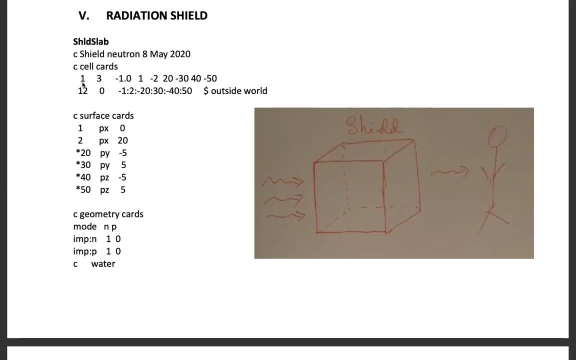 So the first, the shield itself, is cell 1, and it has material 3.. I'll just take you down to material 3.. Material 3 has a density of 1 gram per cubic centimeter, which means it is water. 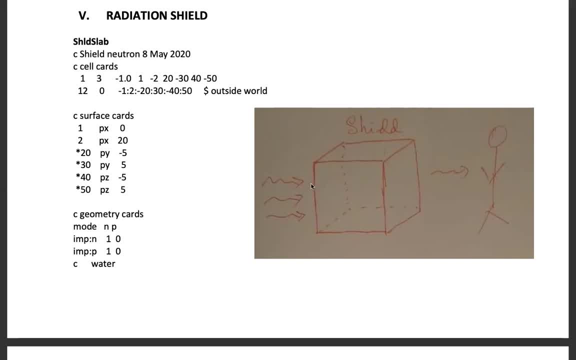 And it is to the right of surface 1,, which is this, left of surface 2,, which is this. So it's between these two. in x, It is greater than 20 and less than 30. in the y direction, It is greater than 40 and less than 50 in the z direction. 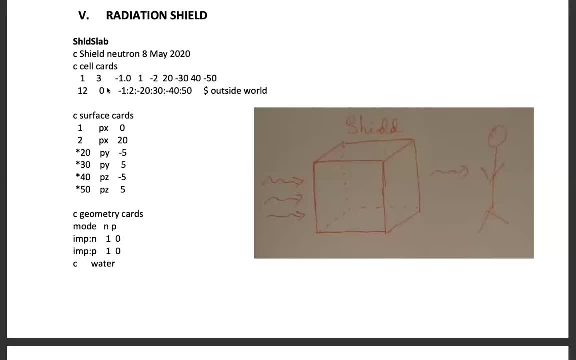 The outside world is cell number 12. With nothing in it, with a void in it, So I'm not interested in air. I'm going to call it void. Of course, in real life you'd have air and humidity, so you need to bottle it with real life conditions. 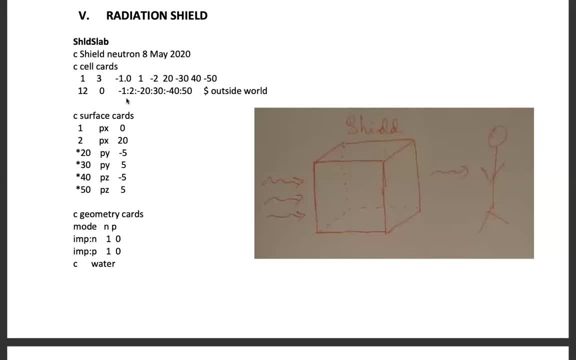 For the time being, let me just say that there's nothing outside. Again, this is a non-reentrant surface, which means that once radiation is left, it's not going to come back over here. Okay, so this is the outside world. 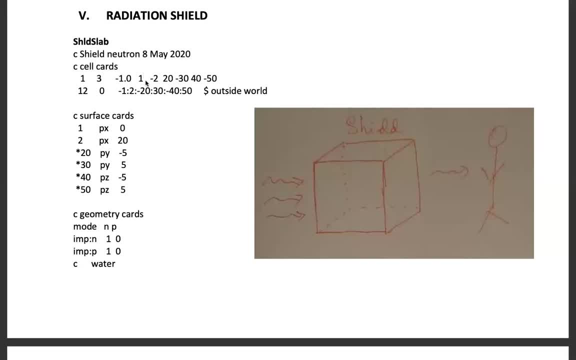 The outside world is opposite of this. So if this was greater than 1, this is less than 1.. That was less than 2, this is greater than 2.. So all the signs over here are inverted over here. So it's the outside world. 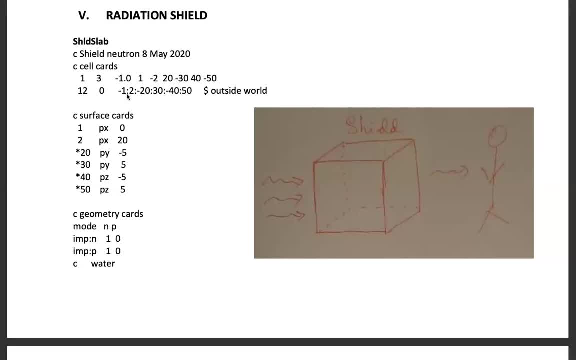 And there is a union operator. So when you don't have any Boolean operator here, that means the intersection. So this is the intersection of everything to the positive of surface 1.. With that of negative to surface 2.. So this is the union of everything less than surface 1, everything greater than surface 2,. 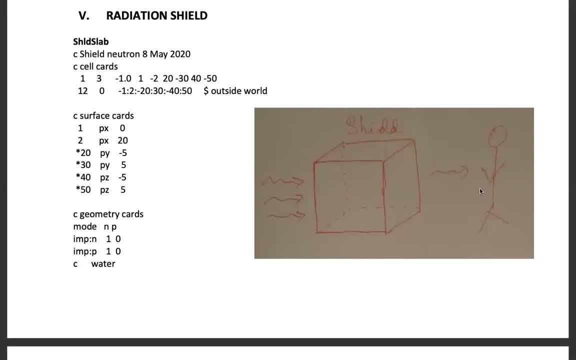 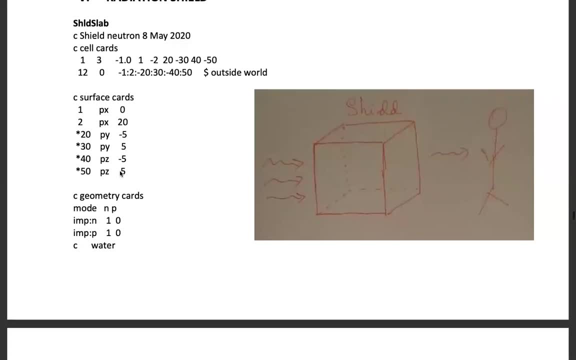 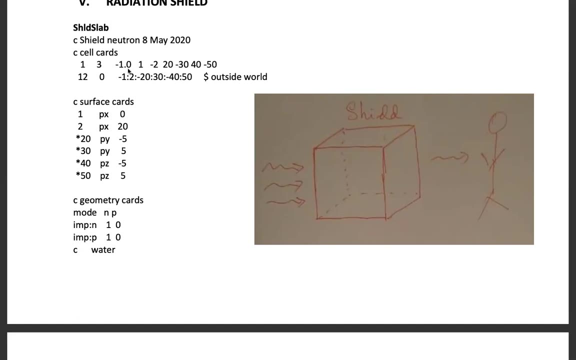 everything above this, everything below this, everything in front of this and everything behind it. So that's what we call the outside world, Now the surface cards. also, let's look at the geometry. Now we just have one material, which is material 3,, which is water, with a gram density of 1 gram per cubic centimeter. 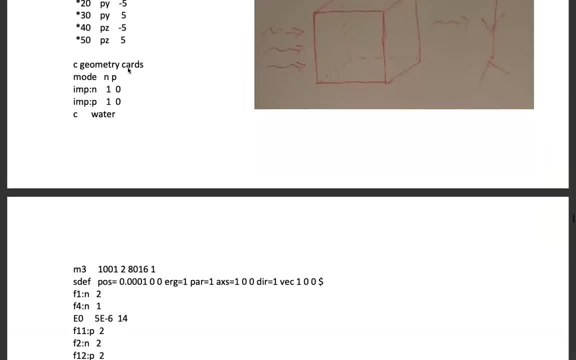 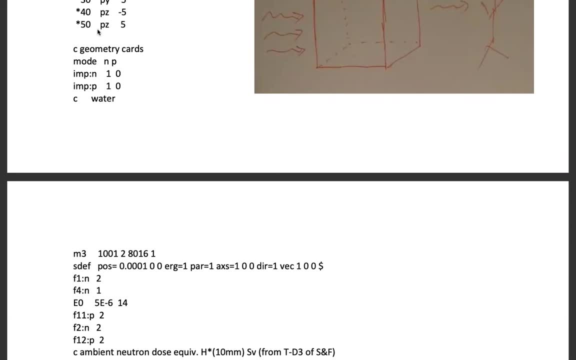 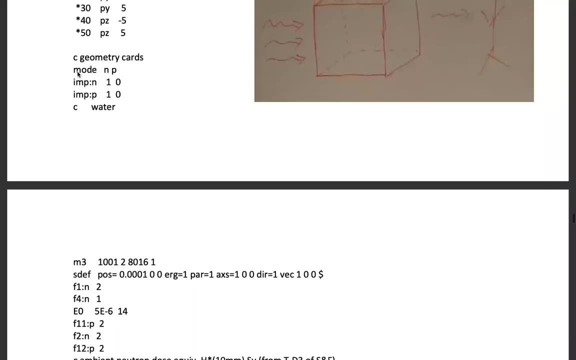 All right, Okay, now let's look at the third. So these geometry cards were supposed to be this label they're supposed to be to. It's a comment card, so it doesn't make any mistake to my simulation. Okay, so it's a neutron photon problem. 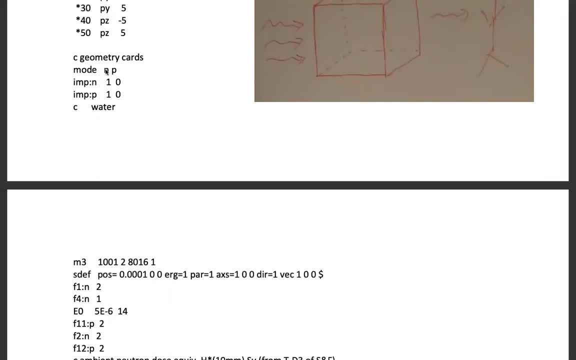 Why? Because I've got a neutron source, But those neutrons can generate photons And I don't have a neutron source. But the neutron source can generate an electron can generate photons And I don't have a neutron source. want to kill the photon when it's generated. so i want to do combined neutron and photon transport. 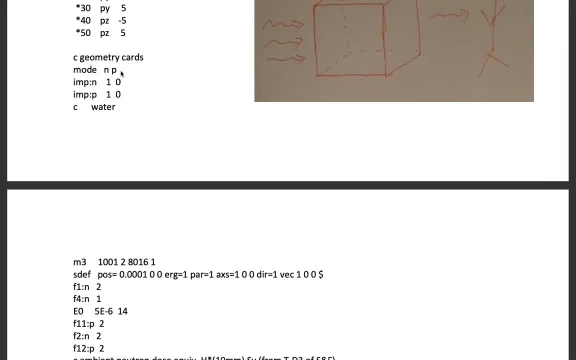 now mcnp can also do an npe- neutron photon and electron- but right now let's just do a neutron photon problem. the two importances i set for neutrons: one inside the shield and zero outside. so one zero, one zero for photons, one zero for neutrons. okay, now this is the material three. 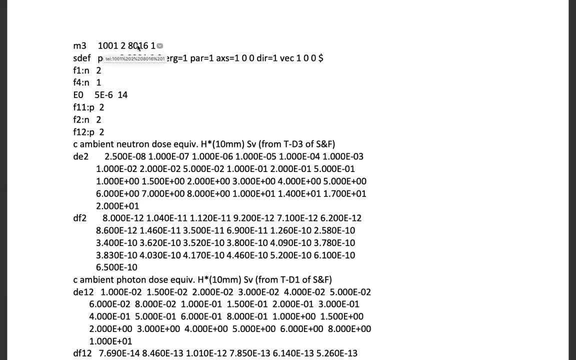 that i'm going to use material. three is h2o. again, i've not said i'm not specifying the cross-section library, because i'm letting mcnp select its own default value for the hydrogen cross-sections and for the oxygen perception. okay, now let me define my source. i say that the position is x. 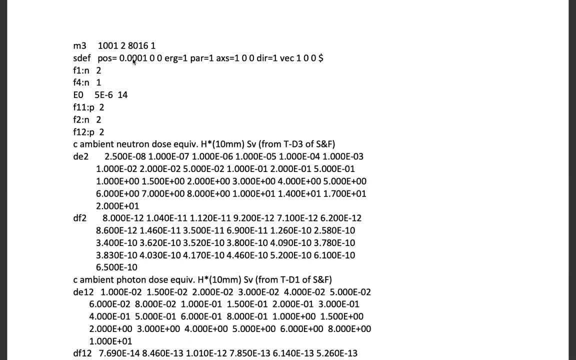 y is that? why don't i take x equal to zero? i can do that, but i just want to take it slightly to the right of the boundary. i don't want it to coincide with about i. i cannot take. i cannot take the source, uh in a, in in a region of zero importance, so i cannot do that. so this is the. 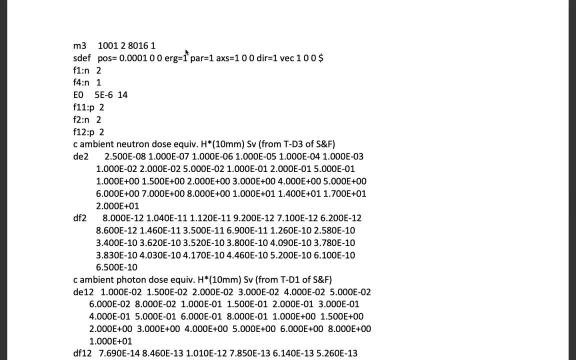 position of the source and the energy of the source is one mev, the particle is a neutron and this is the anisotropic source along the unit vector, along the x-axis. so the direction of the source is here, it's in the vector one, zero, zero. okay, now here's the neutron current. 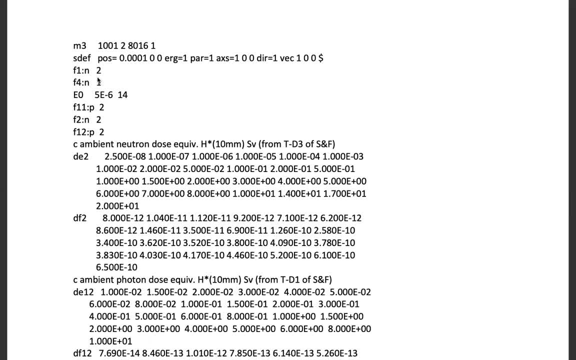 that i'm looking at the neutron current crossing the right boundary of the slab, which is surface two, the flux i'm going to take inside the shield now, here, in the last problem i did not have energy bins, so here i've got an energy boundary of the first result that i'm going to show you will be. 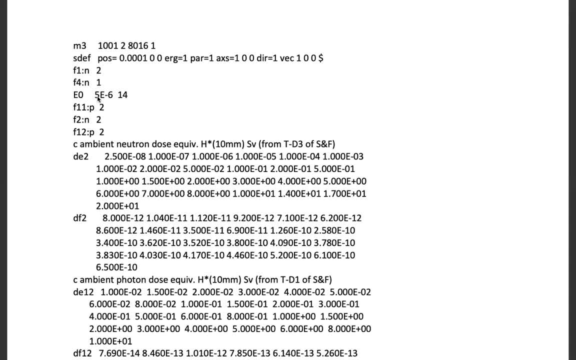 between zero and five ev, and the second i'm going to show you is between five ev and 14, and the source i've got is one mev. so this i've taken as five ev because, uh, all the thermal neutrons and one one ev neutron. 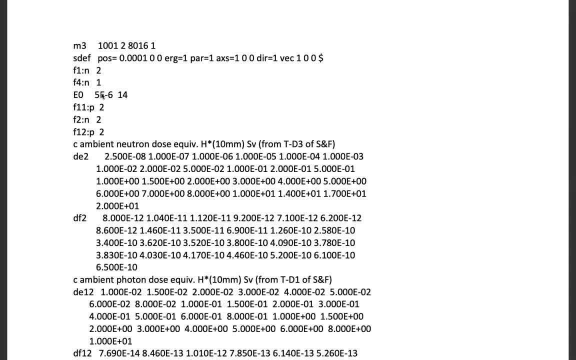 would also be here, so i'll just get a picture of it. so these are the two neutron tallies, the f1 and f4. then i've got- there's also an f2 neutron tally, f2- neutron surface two. then for the photons, i've got a tally type one, since i've used one, so i'm going to call it f11 for a photon surface two. 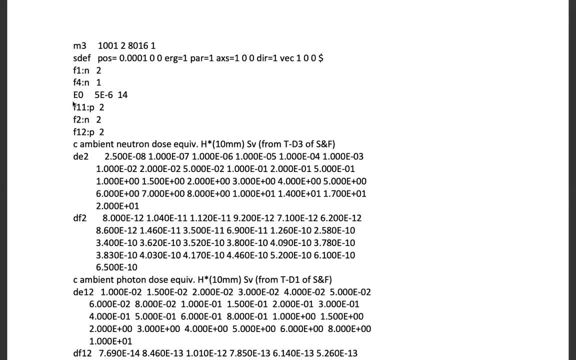 so at surface two, i'm getting the neutron current and the photon now in the cell flux. i've got the neutron cell flux. in one, i've got the. okay, i've got the surface flux of photons on surface two. for neutrons, i've got the cell flux. why? 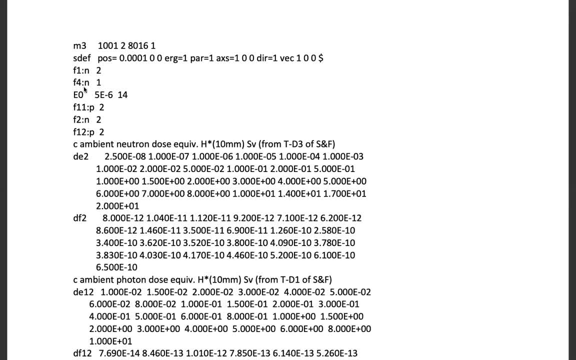 because inside the cell i would also like to estimate a reaction rate. so i need the track length estimator of the flux inside the cell. i'm going to multiply it by the n gamma cross section so that will give me the number of gammas produced by the neutrons. 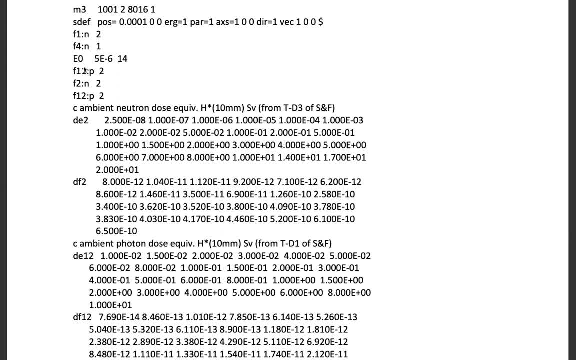 okay, now here are, because i've used tally number two for neutrons and tally number 12 for photons, so i've got to to give my uh, those energy bin values and the flux to those conversion factors. now, these i have taken from uh, from the standard. 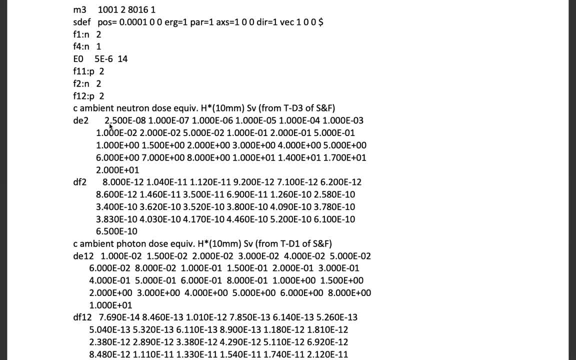 icrp and the bin values are from 2.5 or 0.025 electron volts all the way up to 20 mev, and at those values these are the flux to those conversion factors. now, this is for tally number 2. tally number 2 is neutrons. so what mcnp will do is that it will take the flux and it will multiply. 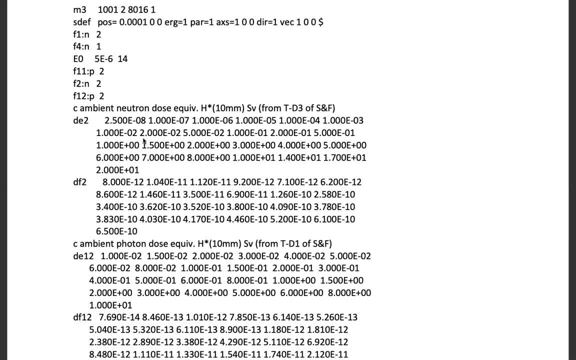 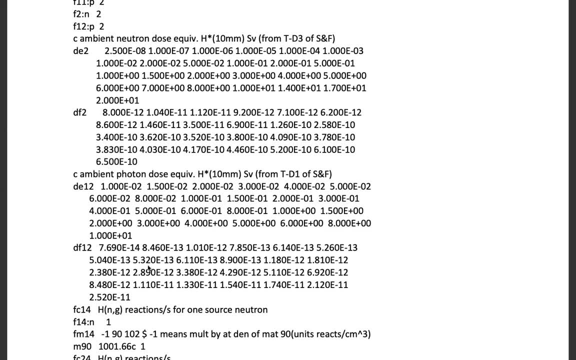 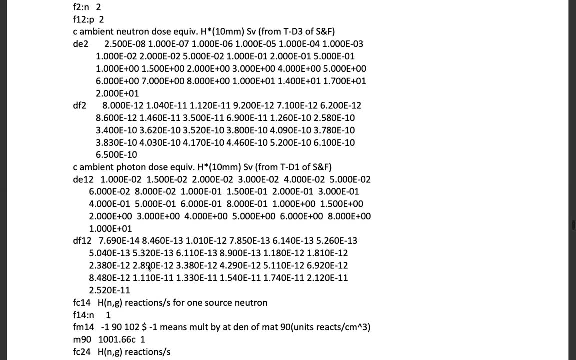 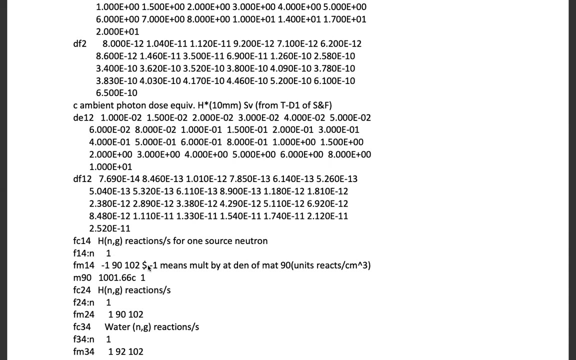 by the n gamma cross section. okay, now same thing for photons. over here this is called the h star, 10 millimeter values. so okay, so that's the neutron and that's the photon. uh, flux to those values. so again, up to tally of tally. n is the ripple vector. so if you get 14Watch, 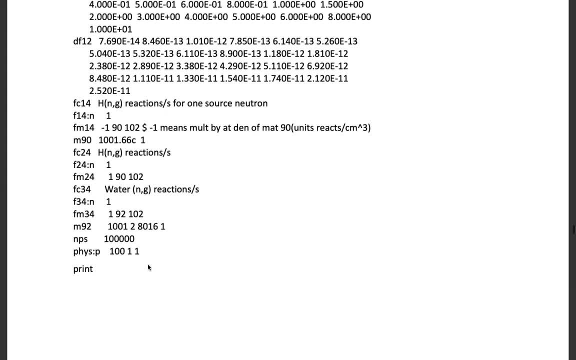 so let's consider a portion of the �on here as a film, and if this is being produced. 14 has three cards, four cards. The comment for 14 is that I'm going to calculate the N gamma reactions, And this is all again for one source, neutron right. 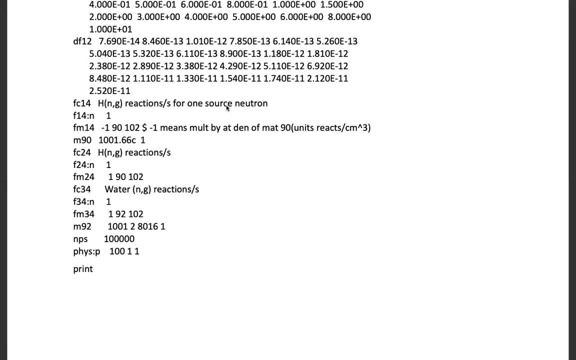 This is exactly what I told you for the Godiva case: that you have got to normalize your results to the actual source that you've got Now here. you can use a californium source or whatever, but you have to normalize your results. 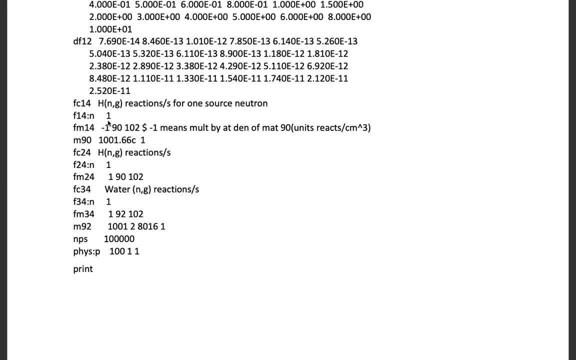 but I'm going to do it for one source: neutron. We can also have the multiplication factor inside over here. We can multiply in FM 14, but I'm not doing that over here. So what I'm doing is I'm giving it a minus one. 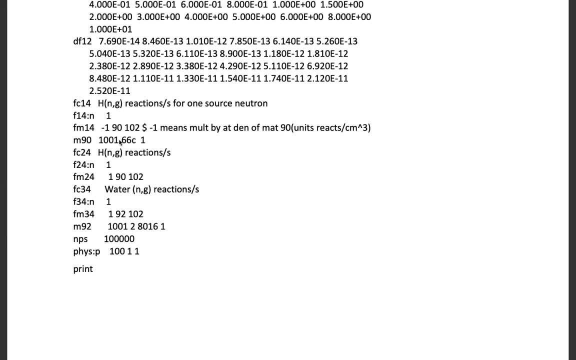 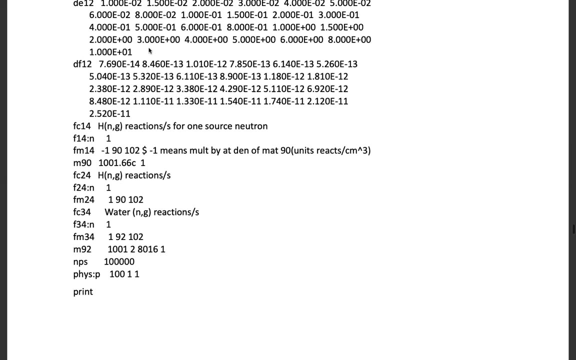 which means that from the problem specified, get the atomic density of hydrogen. And for material number 90, which I have defined separately over here, because this is a hundred percent hydrogen, Previously I defined material number three, which was not a hundred percent hydrogen. 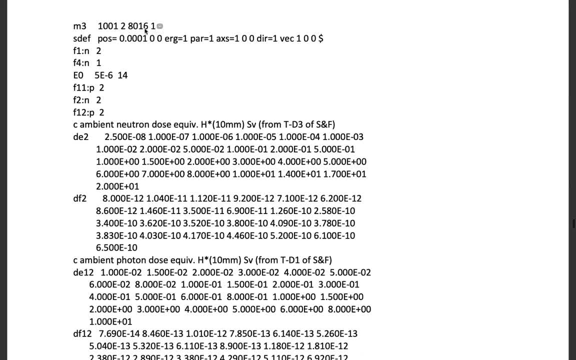 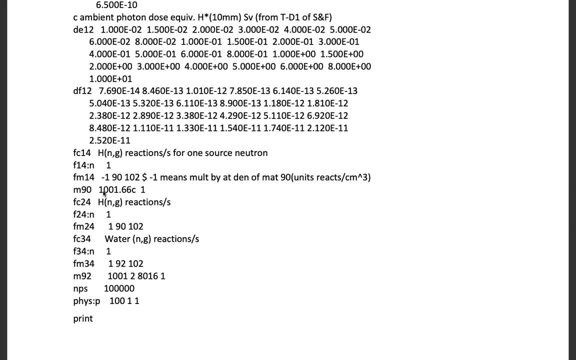 but which was H2O, So I don't want to do it in that. So I define a material, number 90, and the cross section is 1 0 0. 1 for hydrogen, 0.66 C is the library and it's a hundred percent hydrogen. 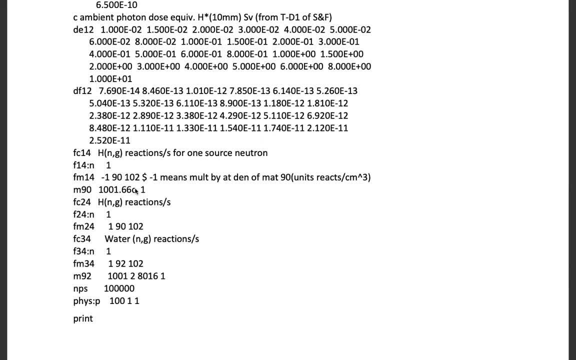 So the reaction number is 1 0, 2.. 1 0, 2 means the N gamma microscopic cross section. Here's the dollar sign, which means that minus one multiplies the number by the atomic density of material. 90 in cell number one. 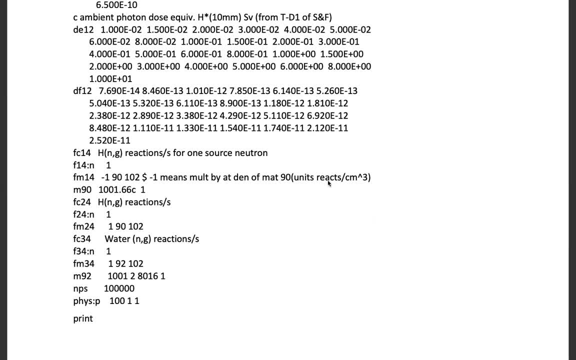 So the answer that I'm going to get from here is reactions per cubic centimeter per source neutron. So that is what Tally 14 is Now. Tally 20 is the number of electrons per source neutron. Tally 24 is the same thing. 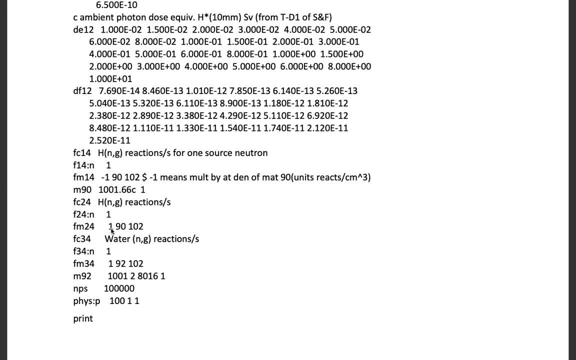 but I don't have a minus one, I've got a plus one. Okay, So here, what you need to do is now this happens in the earliest purposely for you- that first you do it with minus one, then you do it with plus one. 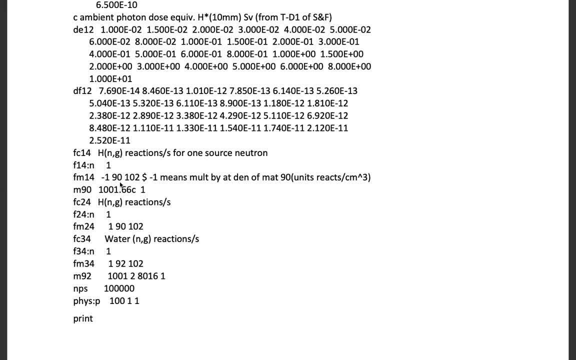 and see the difference in results and satisfy yourself that here it does multiply by the atomic density And here it does not multiply by the atomic density And here it does not multiply by the atomic density. So 14 and 24 are tallies for HNG. 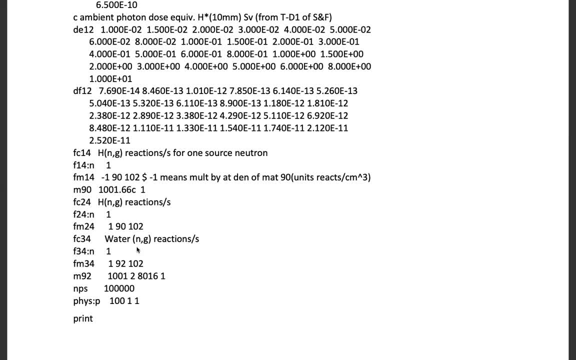 Now let's look at NG in water. Now this also I've done so that you can see that if you define another material called 92 as water, then because there's going to be some N gamma in oxygen, although much less than water. 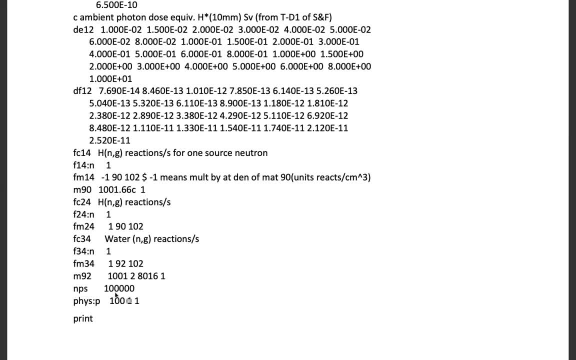 Okay, so I'm gonna take 10,000, sorry, 100,000- histories over here. So the number of particles samples- but here I'm not using the numbers- is 100,000.. Right now I don't know how much computer time it will take, but I don't think. 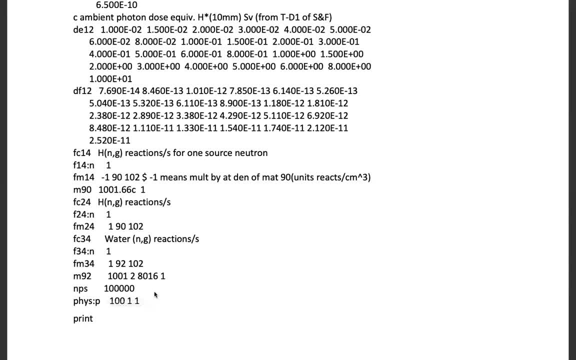 it should take more than 10,, 15,, 20 minutes. So I've just put 100,000.. If you want to specify that you don't want to do a run beyond 10 minutes, you can say: instead of NPS, you can say CTME. 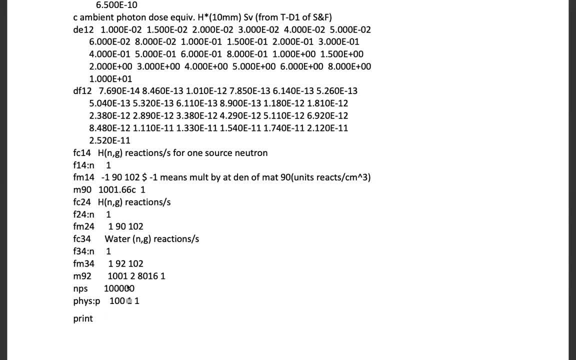 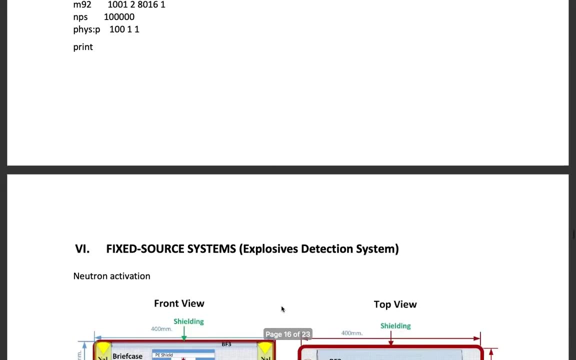 cut me after five minutes or 10 minutes. Now this is a physics card for photons that you don't want to waste too much time and very low energy photons, So you can see that this is the cutoff and this is the print card So you can print your results. Now on the results of the radiation: 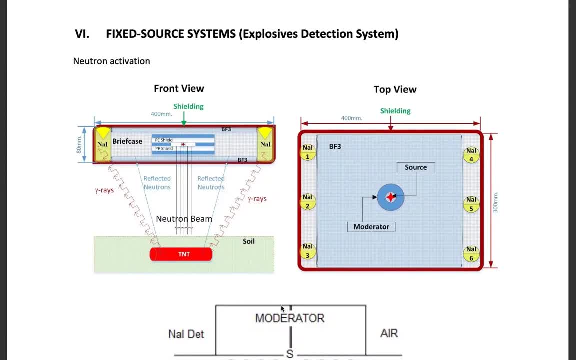 shield. I spoke to you in, I think it was lecture 23 or 22.. So please see the results. Okay, Now let's come to the second problem that I want to take you through, And this is a fixed source system. Again, it's an explosives detection system. 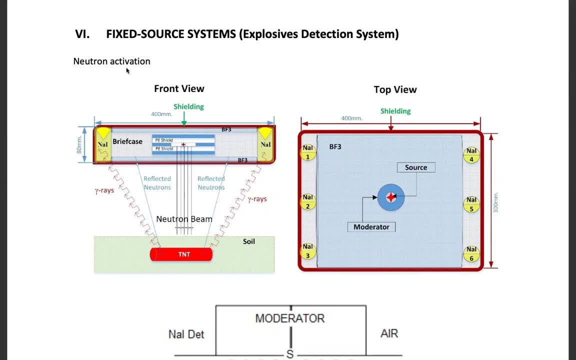 And it's an interesting problem because it is identification of materials. Now, if you are working in NDT, NDT is non-destructive testing, which every atomic energy condition has, and what they do is that they identify materials by non-destructive testing. 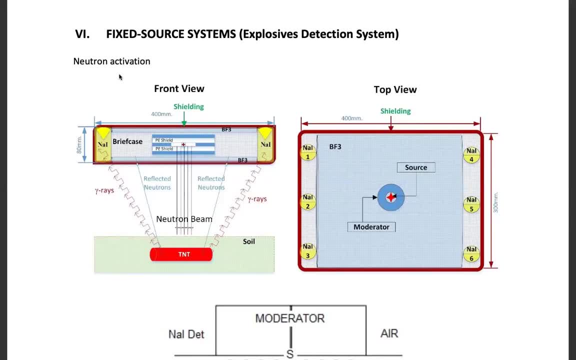 So you do not want to burn vaporized the material and you want to determine what the composition is. This is a field. application of neutron activation. Neutron activation is a field where you fire neutrons and activate something. Now, when a neutron gets, when a nuclei gets activated by a projectile neutron, then it goes into an. 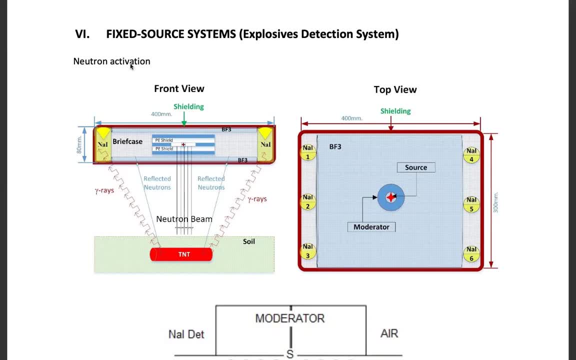 excited state and it can do one of many things, and one of those things is that it can emit a characteristic gamma ray. so if you have a fast neutron hitting something and you carry out an activation analysis, that we call that fast neutron activation analysis, FNA. if you fire thermal neutrons and try to do 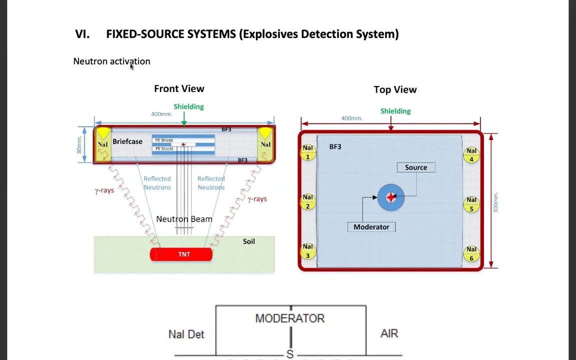 the same thing, then that is called thermal neutron activation analysis. now the problem on the field is if you're going to inspect a bridge made of concrete which is 60 years old and you're going to see if it has cracks, if it has developed cracks in there, so you have to go to that bridge and to fire. 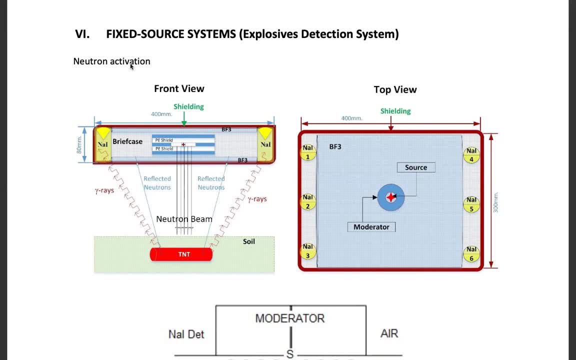 neutrons and you have to get the scattered distribution, the spectrum, and from that you can. you can determine the cracks or you can have a transmission. if you see, the good thing about neutrons is that it is a penetrating radiation. so neutrons and gammas are penetrating radiation. they 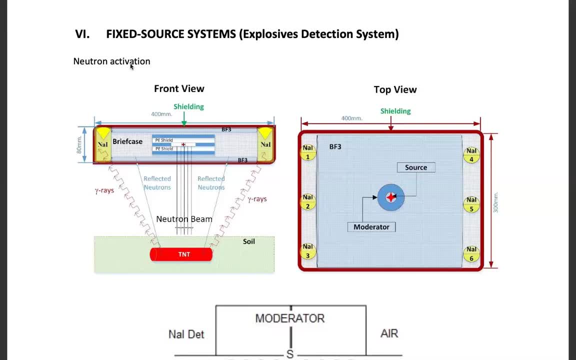 can also go across a solid. now, when we go to a hospital, we are fired with x-rays, because if there is a fracture in the bone, then an x-ray, which is a more energy than a gamma ray, so an x-ray is more effective than a gamma ray. 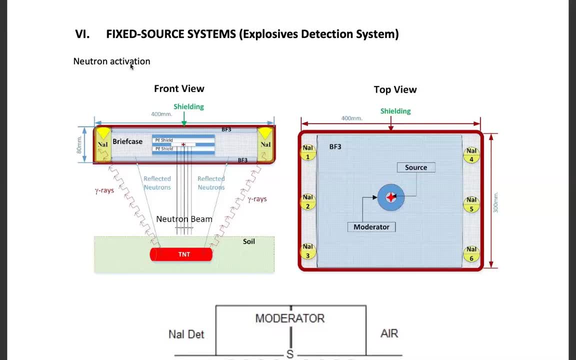 can go through our body and take a picture on the other side and if there is a crack in the bone, if there is a fracture, then you see it in the x-ray film. so now thermal neutrons. you don't have a thermal neutron source, so usually you fire. 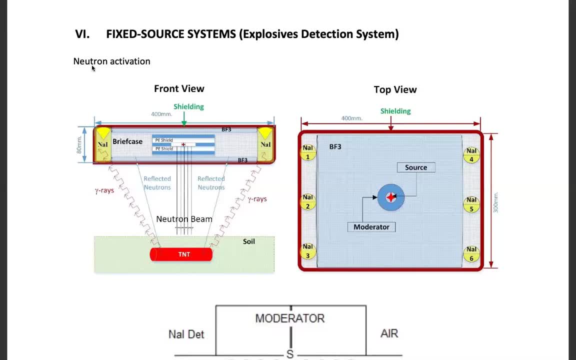 a fast neutron. so this is the study: that in a thermal neutron activation problem, what kind of a moderator do you need to slow it down so that you get a good signal for detection? okay, now, this is an explosive detection system. as you know, many countries of the world where there were wars, 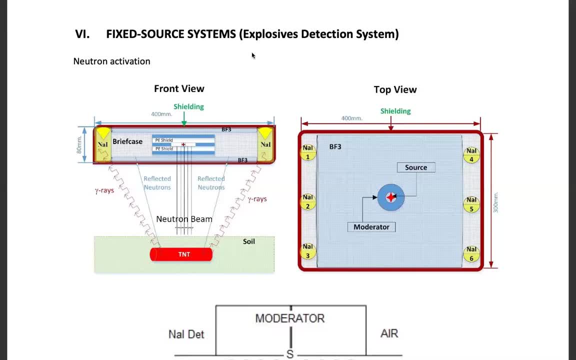 so the armies used to go and lay mines. now mines can be very small butterfly mines. they can be of a few 200 grams. they can be big mines to blow up tanks of the enemy when the enemy is advancing. so these mines are usually hidden under the ground. 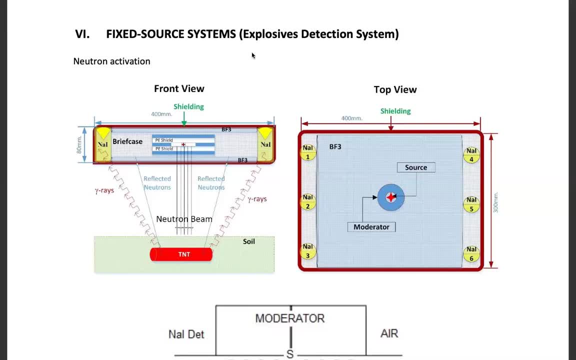 now, after the war is over and the armies have gone, so many of these mines left behind. for example, in Bosnia, in Iraq, in Afghanistan, there are many mines and when children go and play over there, so remember when you were a child you used to go and run and try to. 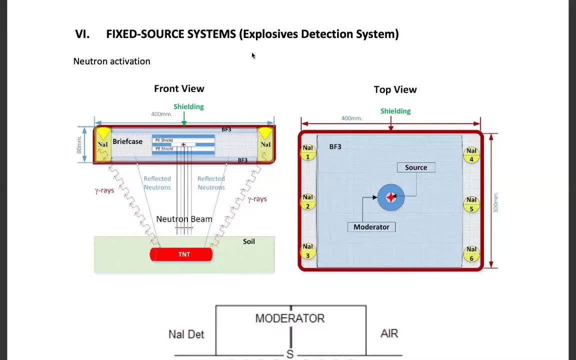 catch a butterfly. so, just like that, little boys and girls, if they see a red and yellow and pink butterfly they go running and get excited and catch the butterfly. and that turns out to be a mine left by some army 10 years ago so it can kill them. 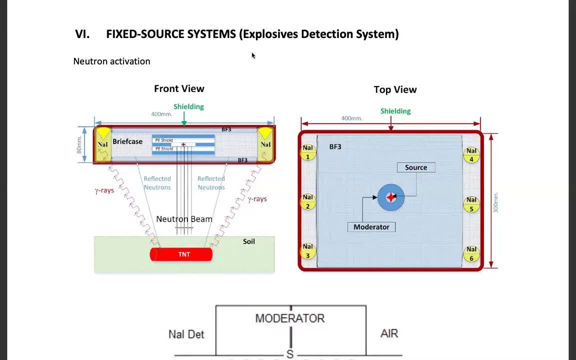 it can blow up their feet and hands. so this is a it's a humanitarian effort to design small detection systems which are portable, which you can scan an area where a war has taken place, and it would be very nice if you can demine the area so that it is clear for children. 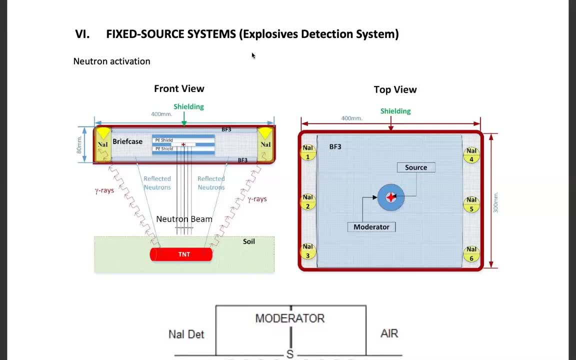 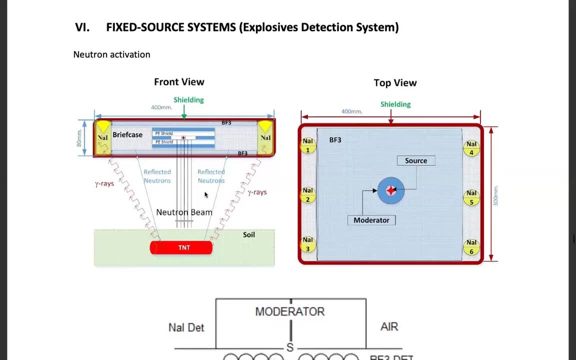 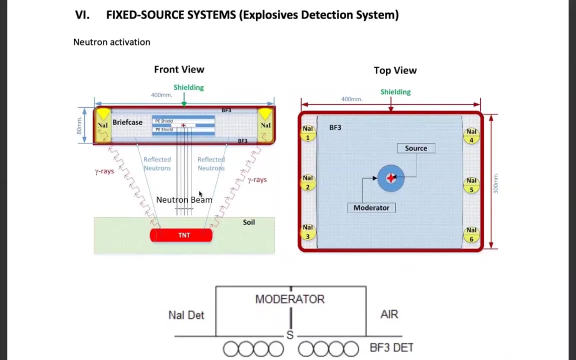 and for human beings to just live over there and grow crops over there or do whatever. so here is a study. again, this was a PhD study. there's a paper on it by Hamza Khan myself. so okay, so this is the front view of a briefcase. 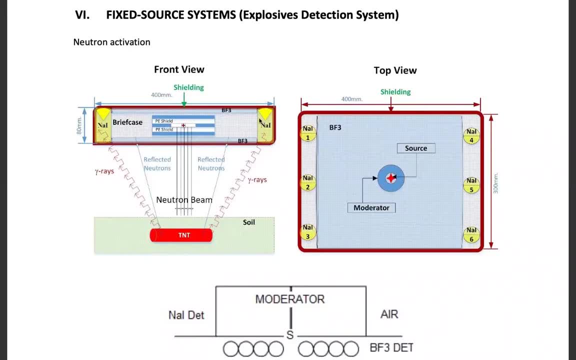 so you can see that this is like any Samsonite briefcase and we've got a source over here. so the source and the source of the briefcase: there's soil. we're walking over some soil and, let's say, under the soil there's some explosive which is hidden away. 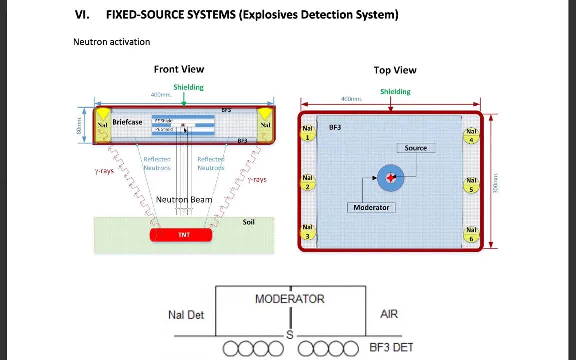 so that I've colored red over here. so if you fire a neutron beam, a fast neutron beam, so it activates the explosive if there's an explosive. if not, then if there's rock or soil, anything, okay, it activates it and what you get? you could get gamma rays coming out of it. 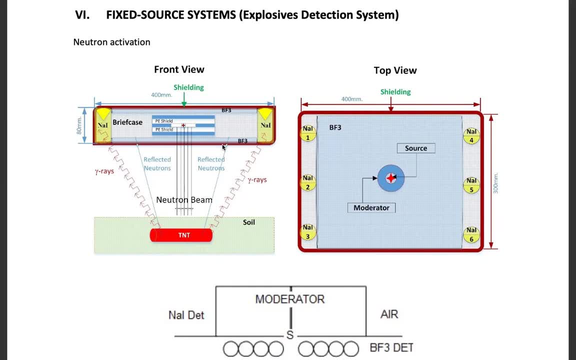 you could get back scattered reflected neutrons coming and then you can have detectors over here. you can have BF3 detectors. okay, boron trifluoride detectors. you can have sodium iodide detectors. you can have BF3 detectors. you can have sodium iodide detectors. 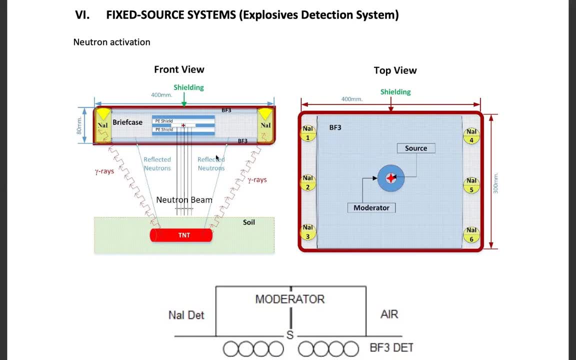 now BF3 detectors are used to detect thermal neutrons because you have a moderator like wax before that and you can produce charge. basically, you ionize the gas and you produce electrical charge and detect the neutrons. now for the detection of gamma rays you can have scintillators. 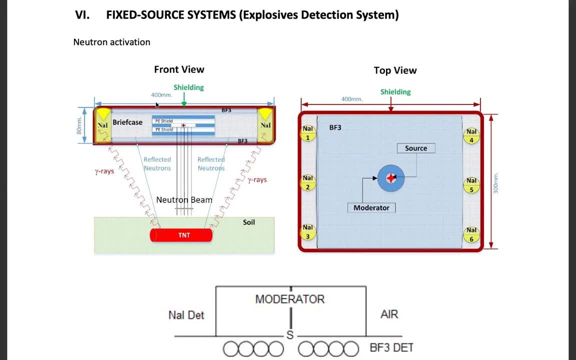 sodium iodide plastic scintillators. so in this portable detection system we've got a source, we've got a polyethylene shield, as we studied in the earlier video. we studied in the earlier lectures that when a neutron collides with a hydrogenous material, then the chances of it thermalizing. 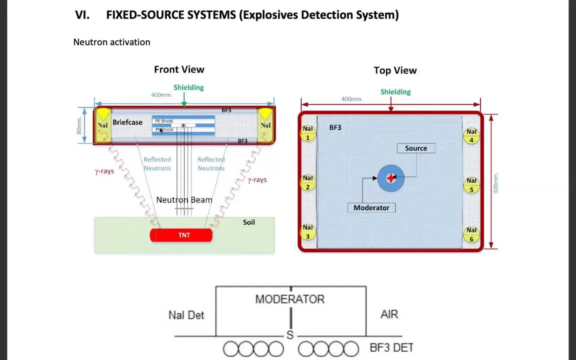 are very good. so here it thermalizes. there's a reason why we wanted to thermalize. I'll just show you. and basically we detected. then you've got your electronics over here you could have a FPGA field programmable gate array and that could be transmitting the signal. 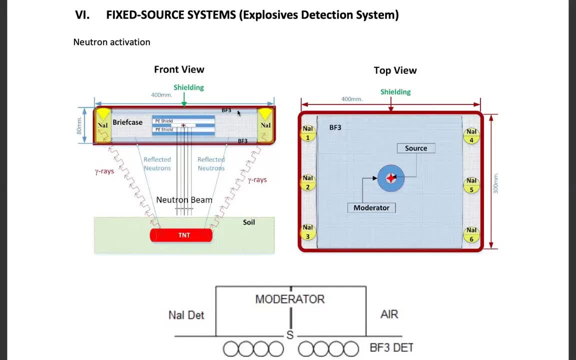 from the field that you're scanning, maybe to a small remote control unit helicopter, and you have to now work out the scan time necessary. can you cover one square kilometer and how many minutes would you take to do so? that's the front schematic of a fixed source explosive detection system based on. 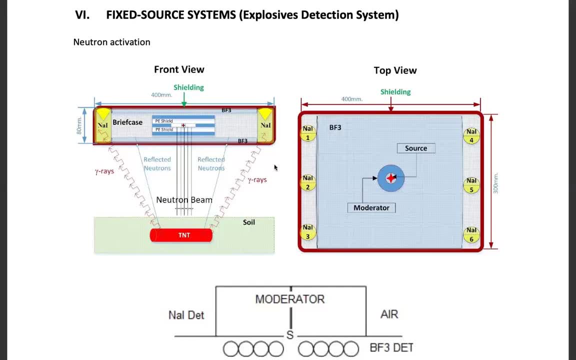 thermal neutron activation. now let's look at the same thing from the top. so here we've got one, two, three, four, five, six little sodium iodide plastics into the detectives and from the top you can see that this is the shielding, this is the source, the moderator: why do we need a moderator? how much moderator do? 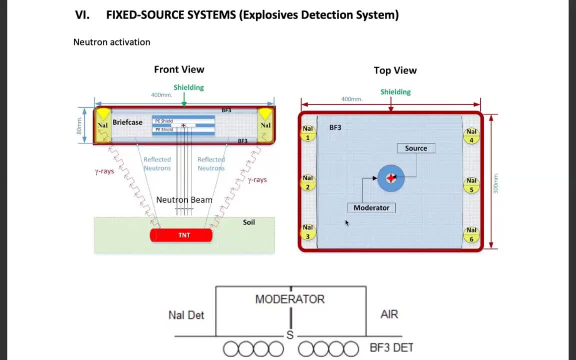 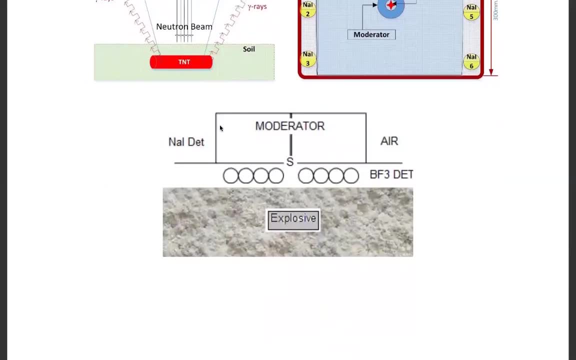 we need. how much shielding do we need? now, all these are the design calculations that you need to do in nuclear engineering. now here's the picture that them are system is going to be sitting on top over here. we've got glass tubes over here and we have a bf3 detector. okay, so we've got a moderator source. we've got. 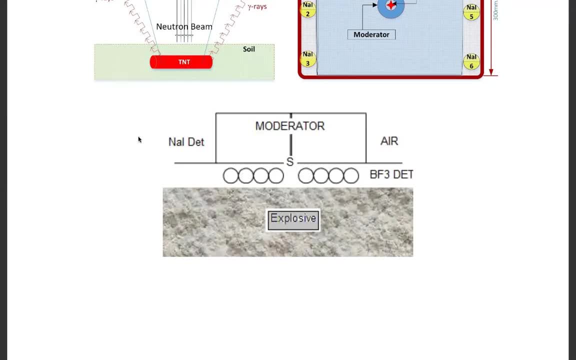 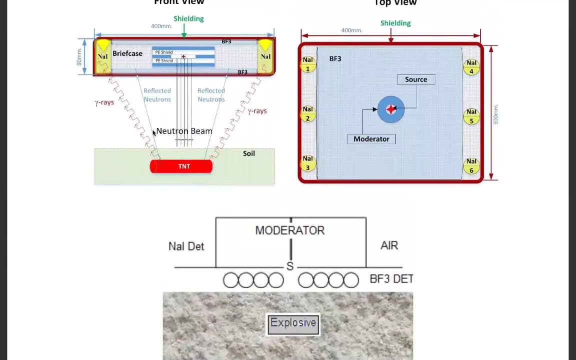 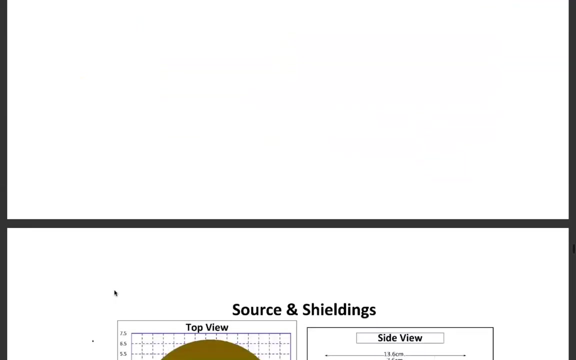 bf3 tubes and the explosives sitting in the ground. so these are the detectors. so let's see how we would analyze this. so we've looked at nuclear assemblies, we've looked at a nuclear reactor, we've looked at the shielding. now this is another nuclear application of non-destructive testing. this is another picture of it. 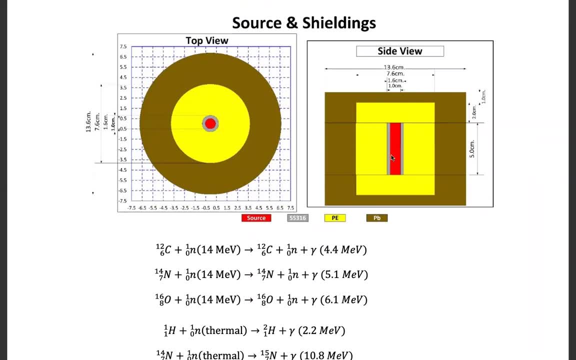 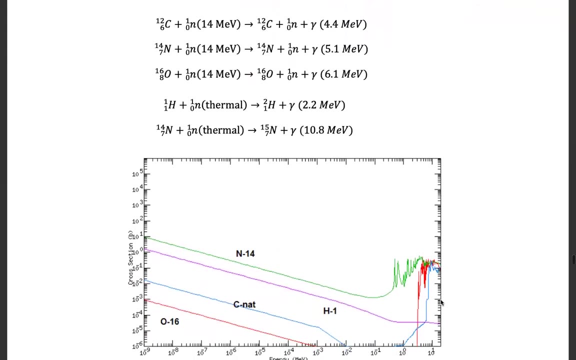 with a little bit more detail shown on how you're going to place your source and what are the dimensions of the source casing, the top view and the side. now these are the reactions. okay, so let me show you the reactions and the cross sections. so, again, before you do a simulation, you've got to understand the 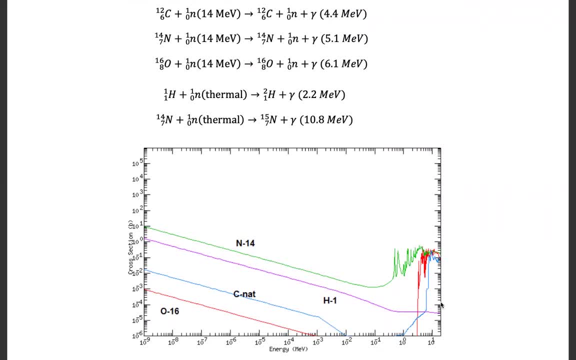 problem. so let's try to understand the problem over here. the problem is the that an explosive like TNT is made up of four things: carbon, nitrogen, oxygen and hydrogen. so I'm going to be interested in these four. of course, these four things are in wood also and there in many plastics also. so you and there in 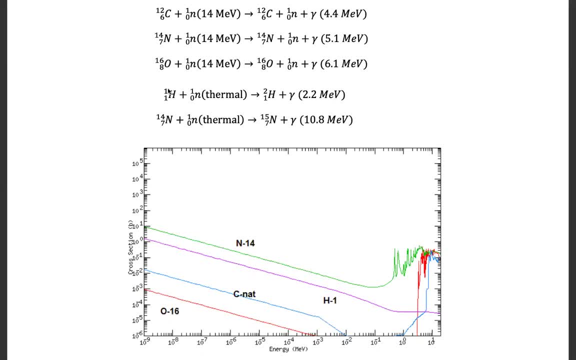 drugs also. so how would you, how would you differentiate between wood if something like this is made up of 4 things? and the other thing is that the is taking a plastic plate in their suitcase. Second person is carrying drugs in the suitcase. Third person is carrying explosives in the suitcase. Now you've got a scanner over there. 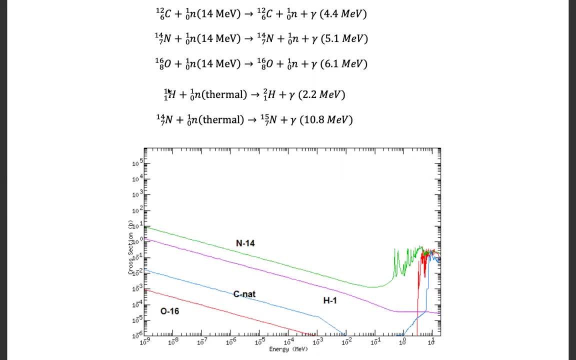 and the scanner goes and when your suitcase goes on the on the belt in the airport, then it's scanned and they want to know from the security point of view, that what is inside your baggage. So this is very useful. at an airport, at a shipping port, at the entrance of a city, You can have all the 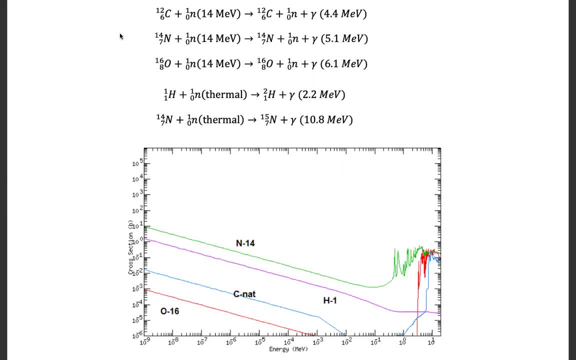 cars that are entering the city, they go through the detection port. So now, if you fire neutrons. so these three reactions are: if you fire fast neutrons, what happens? and these two are: if you fire thermal neutrons Now, so if you fire a 14 MeV neutron on carbon, then it produces a gamma of 4.4 MeV. 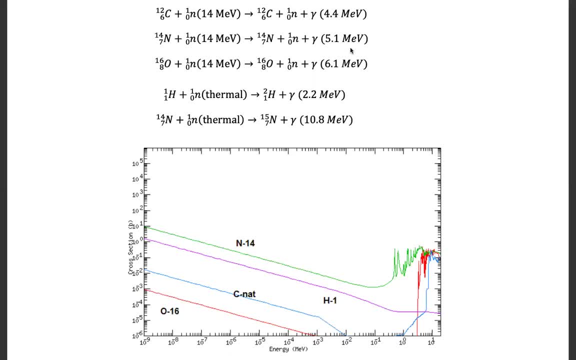 if you fire on nitrogen, it gives you this. If you fire an oxygen, it gives you this. If you fire a thermal neutron on hydrogen, it gives you a characteristic gamma ray of 2.2 MeV. If you fire nitrogen, it gives you a characteristic of 10.8 MeV. 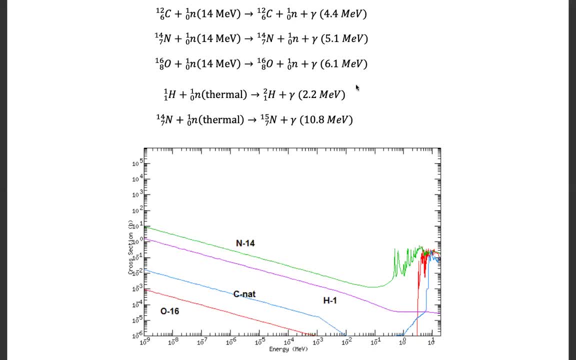 Now, apart from knowing these nuclear reactions, it is also important to know how many of these reactions will take place. So for that you need to go and see the cross-section which I've plotted over here. I've taken this from KAERI, the Korean Atomic Energy Research Institute. 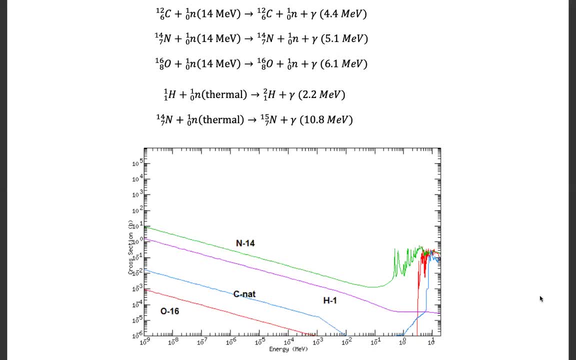 website where they allow you to access cross-sections, to plot them and to define the energy windows, the y-axis, to color differently, and then I labeled this. I transferred this into MS paint and then I labeled it So you can see that the red one is oxygen. so it begins over here and comes out over here. 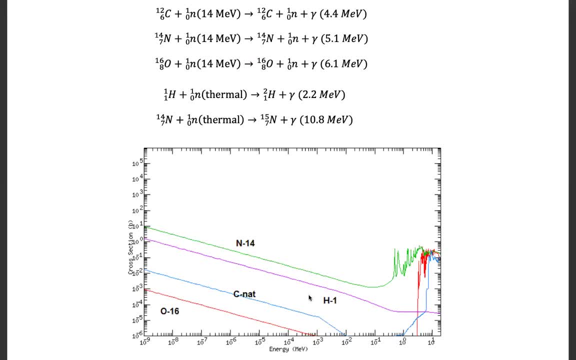 The blue one is natural carbon, the purple one is hydrogen and that's nitrogen. Now for nitrogen. you begin to see a few resonances over here for oxygen and nitrogen. The important point is that this is a log scale and you can see that most of the reactions are going to take place at lower energies. some of 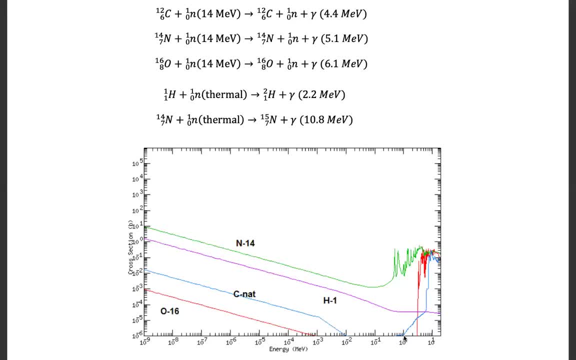 course over here. So, yes, the reaction rate goes up after about 4 MeV and goes up at thermal. so that is why we would prefer thermal neutron activation over here. So let's carry out a study and you can see that the most you. 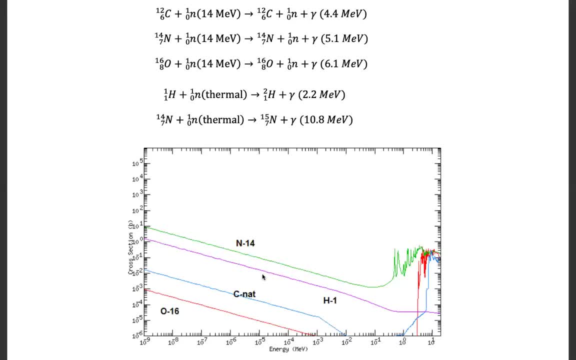 would get is from nitrogen, second, most from hydrogen, while from carbon and oxygen 16. from oxygen 16 and carbon 12, hydrogen 1 and nitrogen 14.. You'll see the most from here second, most from here third and fourth, but these are log scales. 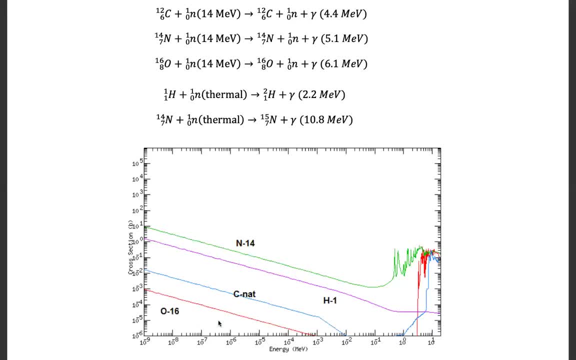 So you will receive minimal signals from over here. but in this Monte Carlo simulation, what do we need to do? We need to model our source, we need to model our detector, we need to model the soil and we need to look at how many grams or 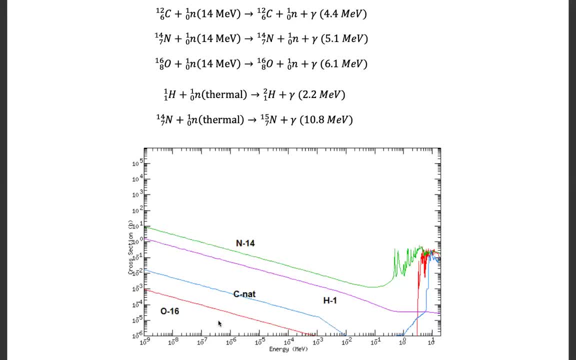 kilograms of explosive are concealed. how many centimeters deep within the ground can we detect the signal? can we, first of all, can we detect it, Second of all, that, having detected it, can we get the chemical formula of the thing that is hidden? Because we want the chemical formula, we want the ratio of the atoms. 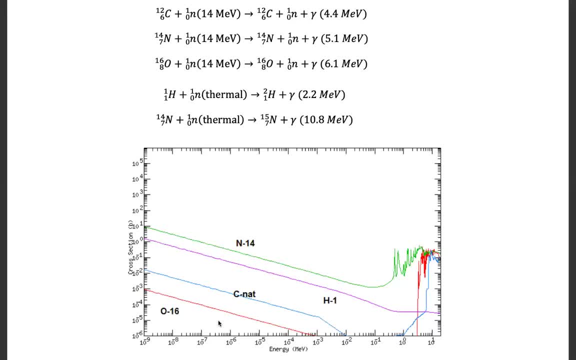 of nitrogen to hydrogen and then in our FPGA we could have a lookup table. you could match your results with the database that you've got and immediately you can say that this is TNT, this is RDX, it's nothing you know, you can, you. 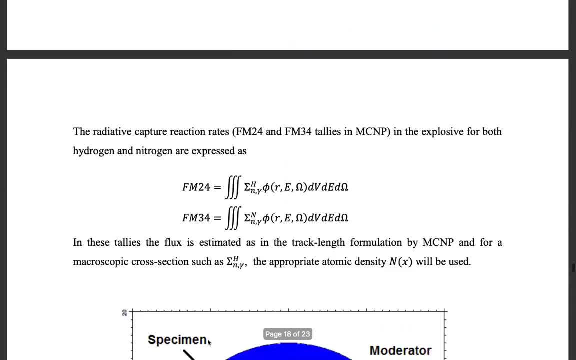 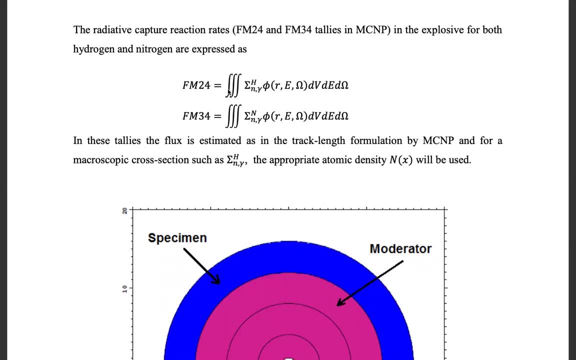 can immediately identify that. You can identify within seconds what it is. So here is our tallies, which I showed you, which we are going to do now. So let's define the tally number 24, the multiplier, tally multiplier 24.. So I'm going to find the flux and see how many variables there are. 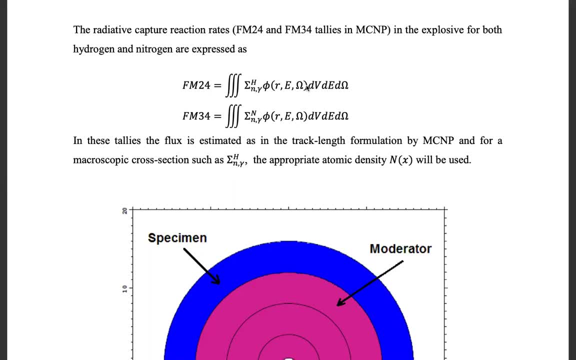 This is the phase space 3, and 2,, 5 and 1, 6 variables I've integrated over time. it's a steady-state problem. So when we started this series of lectures I told you that there are seven variables, but now we've got three and one, four and two six. 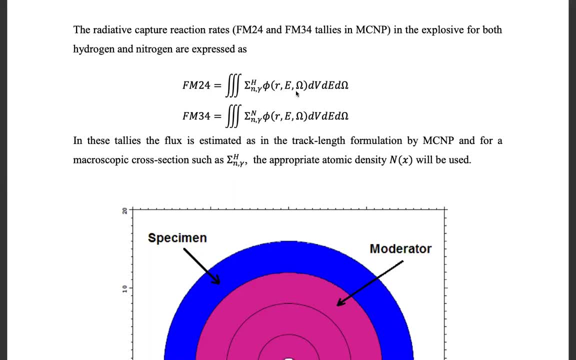 variables, So six variables. can you imagine doing this with anything else other than Monte Carlo simulation? So we are going to get an excellent spectrum of flux over here. We are going to multiply it by the microscopic n-gamma cross section for hydrogen, then for nitrogen. We are going to multiply by the number. 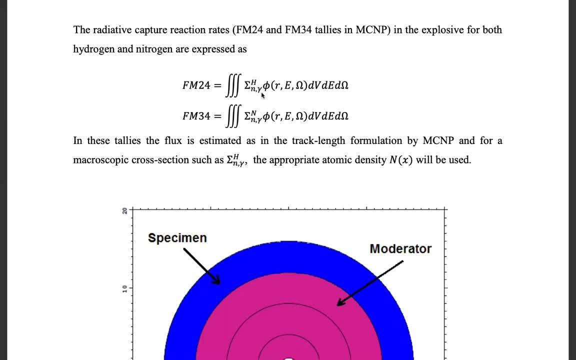 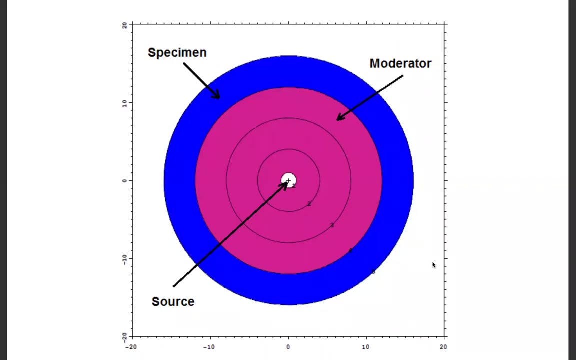 density and we're going to get the number of gammas which are coming from hydrogen and the number of gammas which are coming from nitrogen, and then we will see the spectrum and do our analysis Now, because you saw that the cross sections are favorable for thermal, so this is a 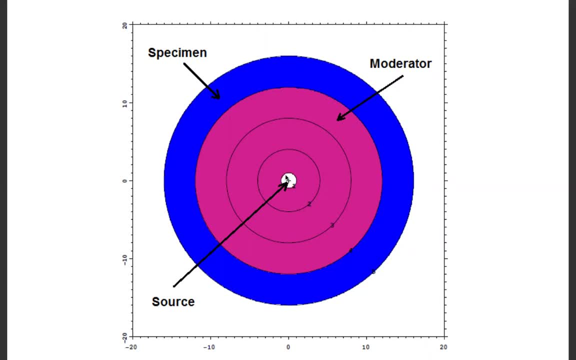 little lab experiment that you should do: simulate that put a source, and here's the blue one, is your specimen of explosive. and what I told my student, my PhD student, to do was take some layers in between and just carry out simulations to see which moderator and how much of it. for example, is graphite good, is water? 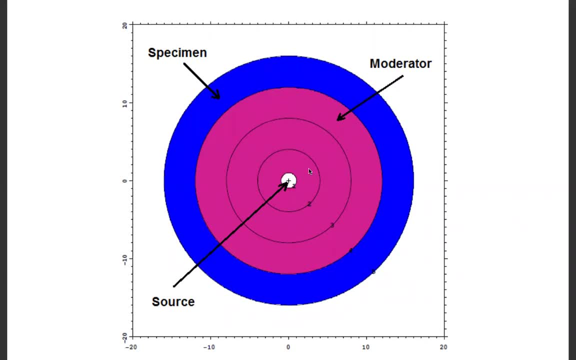 good is wax good? is polyethylene good? what is a good moderator and how much of it do you need? what will be the weight of the moderator so that you maximize the n-gamma reactions here, because outside over here are going to be your? 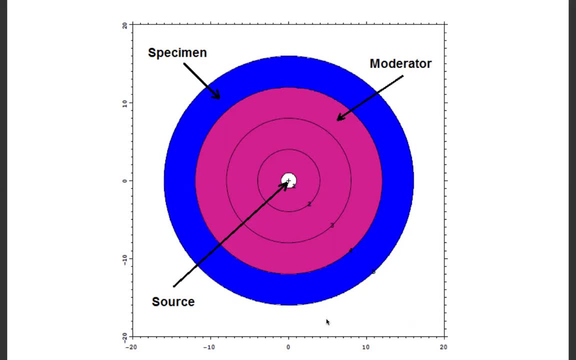 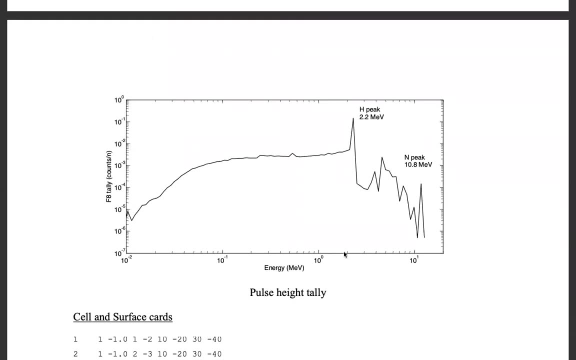 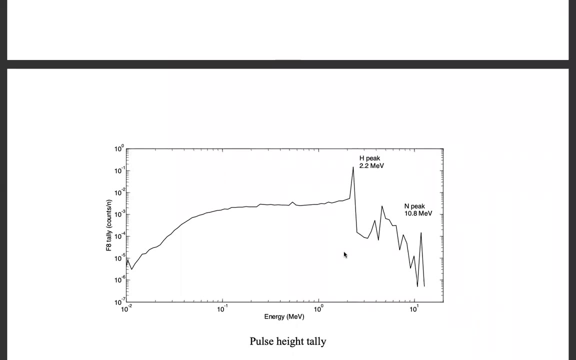 detectors, and you don't have an infinite number of detectors, so you're not going to be able to measure hundred percent of the signal. Okay, so what do we want at the end of the day? We want the pulse height telling, because this is the connection between people like us and the experimentalist who's sitting in a 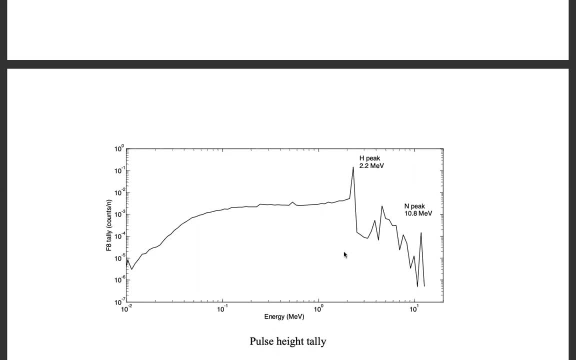 lab and he or she has is going to see something like this, but they've got windows of energy and they're seeing counting the peaks in each, each bin, and so this is my nitrogen peak, 10.8. this is my hydrogen peak. so what I have to do 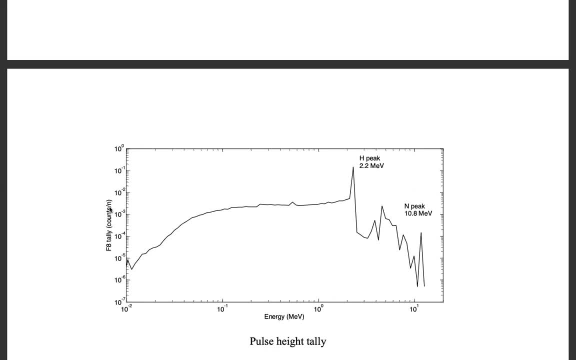 in a simulation is to see how many number pounds do I get from hydrogen, how many do I get from nitrogen? then there are other factors which need to be considered, like the detector efficiency, the solid angle and so on. so it's a big study. but what you need is the f8 tally over here, which Monte Carlo does have. so 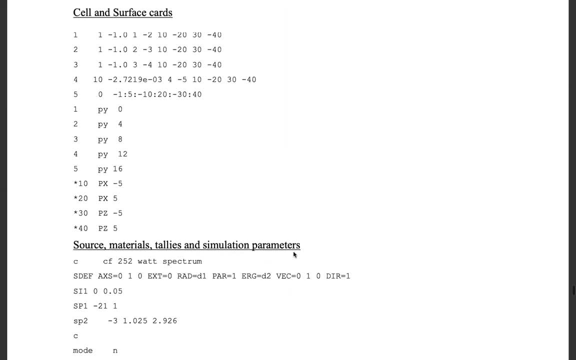 I'm going to put that in the input file that I'm going to show you. so this is the input file that. now you see the number. so this is block one is from here to here. sorry, there should be a space over here, so just to show you a word. 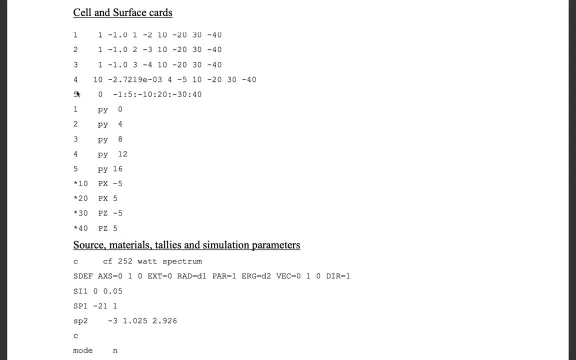 file to remove the space. but this is block one coming from one to five. these are the five cells and the surface is the n-gamma reaction. so this is the second block, which are from one to four. I forgot to tell you in the last input. also add stars over here. whenever you put a star on a surface, that means it's. 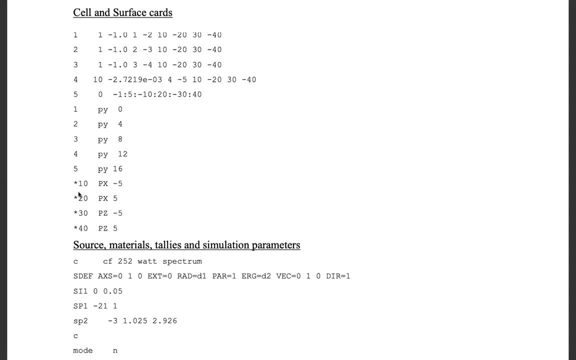 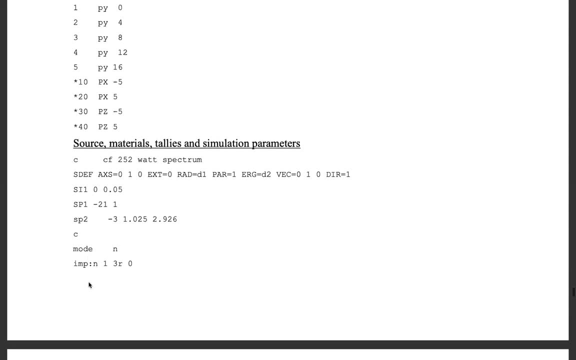 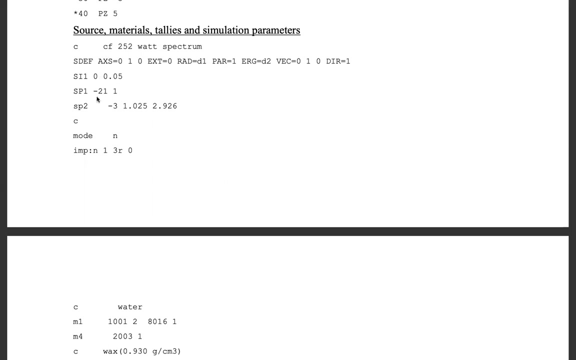 a reflecting surface. so this is the kind of reflecting surface of any neutron going out of there comes back the source. I am using a CF 252 source source, so I use a standard built-in. the source probability distribution is called minus 21, so the source probability, the energy, is distribution 2, so it's SP 2, which is a minus 3 source. 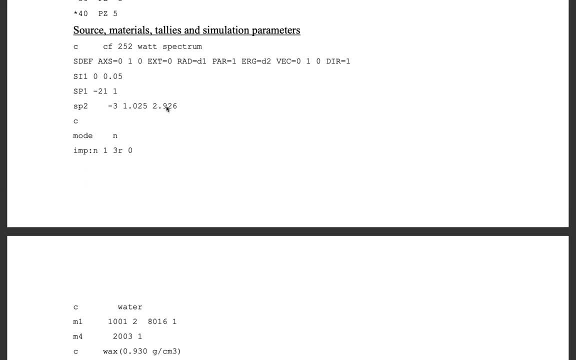 and these are the a and B parameters. if you go back in the lectures, you'll see that these are the parameters of efficient spectrum of CF 252. now, okay, so it's a. this is the definition of the source. it's along the y-axis and I'm going to sample the radius of the source from distribution 1. 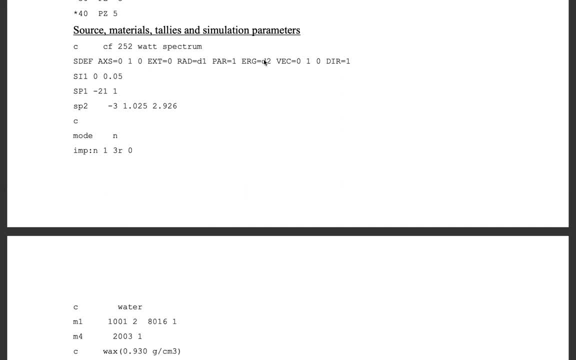 it's a neutron source. it has an energy distribution 2 which I told you about. it is traveling in the y direction, okay, and it said it's at 90 degrees to the X and Z. the distribution 1 for radius, it's going between 0 and 0.05 centimeters and 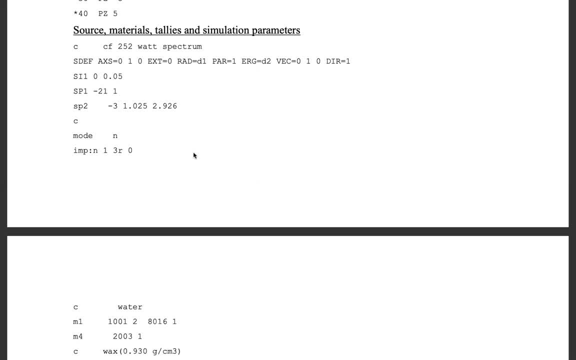 this is a distribution, parabolic distribution profile. I think. please go and check it so you can distribute things linearly. you can define a PDF, CDF, a histogram or a parabolic distribution. and I think I put: this is the thing that you forget after many years. so I should have put a dollar sign. okay, so this is a neutron. 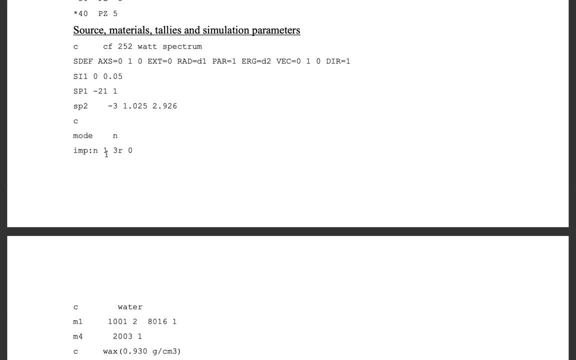 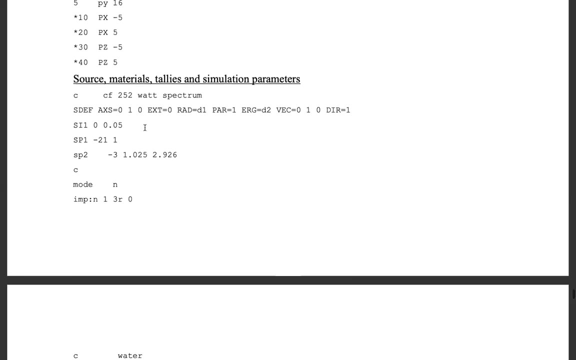 only problem. so it's a mode neutron. I've got one neutron importance for neutron in cell, one in cell two, three and four again. I'm repeating this: one, three times. I got one and three, four and the outside world is zero. so I've got five cells and should be having five cells. so I've got one, two, three, four. 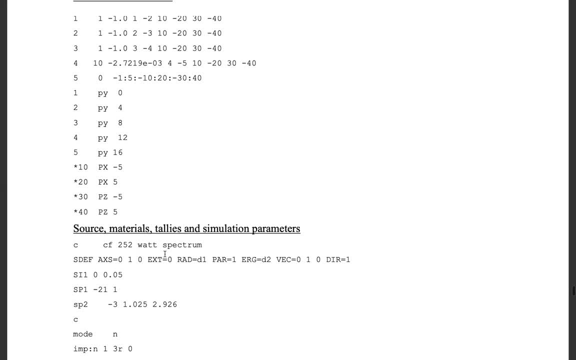 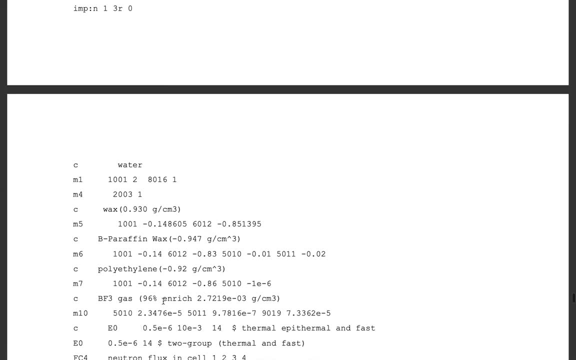 outside world. you see, I should have all comment cards over here, so you should do that. and sometimes, when you have a lot of experience, to say, oh, I know what all this is, but we're all human and we forget after a number of years where it was. 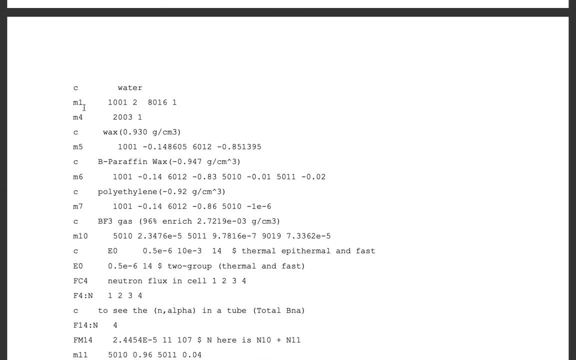 okay, so now let's define the materials. water is material one, h2o. what is this? two, three. okay, so that's helium three. and why did i put helium? i don't think i'm using it here, because some detectors are helium detectors, so maybe i wanted. 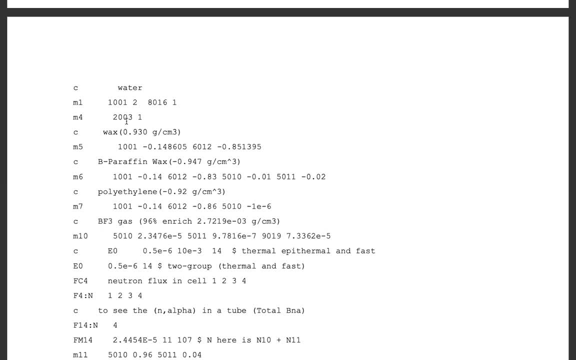 at that time to do a study, that instead of bf3 i wanted to look at a helium detector. okay, now let's define wax b: paraffin, borated paraffin wax- polyethylene. so let's look at three possible moderators now. wax has a density of 0.930 grams per cubic centimeter. this is the composition. 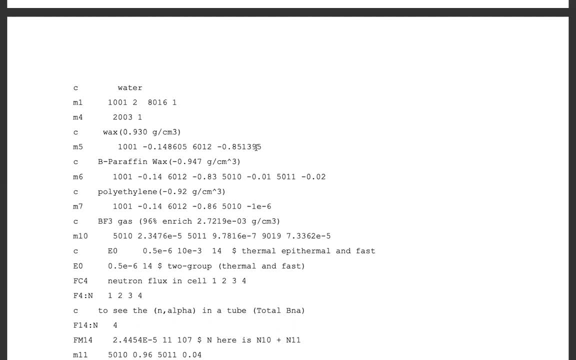 a very nice place to get compositions is the pacific: uh, p and n? l pacific for first nuclear attacks. they've got you can some. it's freely accessible. i use my number densities from there. so from p and n? l you can get your. i think they're called radiation cross. 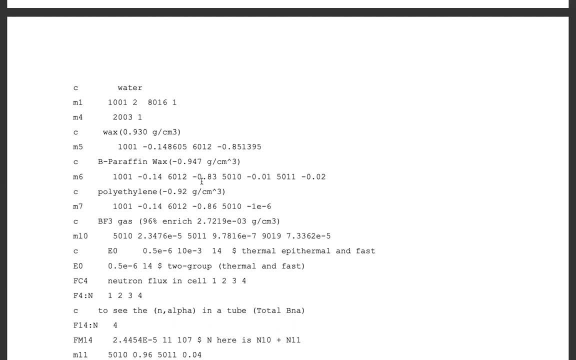 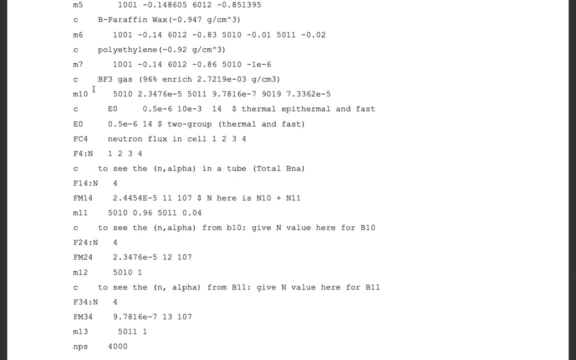 section radiation or cross-section data or radiation compendium of radiation, shielding something. okay, so i've defined material five, six and seven as the three moderators which i'm going to consider. we've got bf3 gas now. bf3 gas in this simulation is 96. 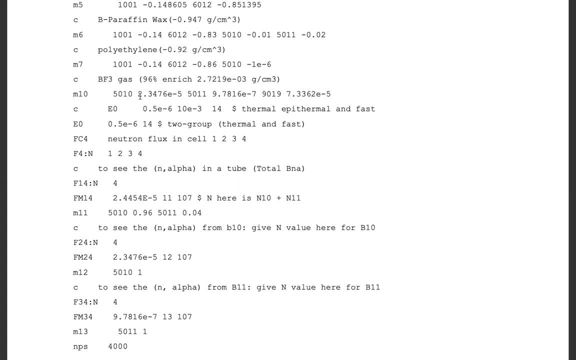 enriched in uh, boron 510, because b511 doesn't have a good cross-section, or n alpha. okay, now the b bf3 detectors. you can study about detectors. they work on the b and alpha reaction, so it's a neutron capture in the boron trifluoride gas, because i had seen these things in the lab where i worked before. 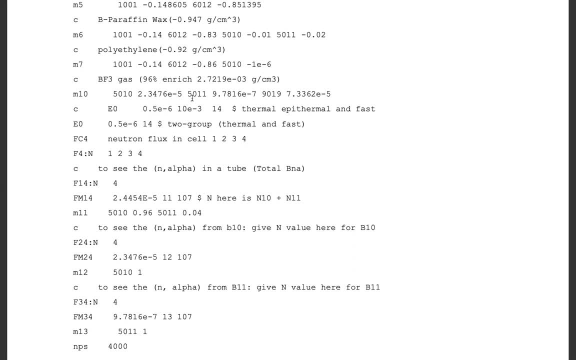 so. so i know that it's a bn alpha reaction is going to take place. so this is the b510, this is the b511 atomic density, this is the fluorine. so you can make, you can study what enrichment you need. but if you have lower enrichment than this, 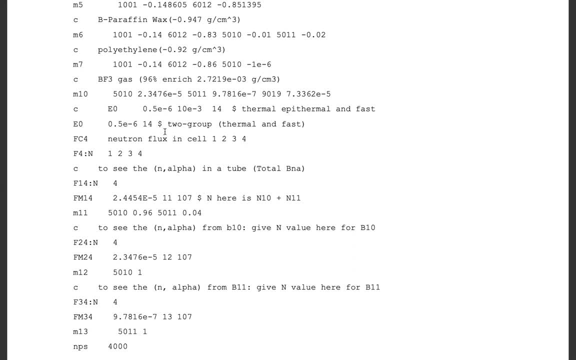 it just spoils your signal. i took an energy two groups as before, and i took the tally f4. the flux tally in regions one, two, three, four. for the n alpha reaction in cell four. this is a tube. so i multiplied by the bf3, by the boron density, i made material 11. you can see is 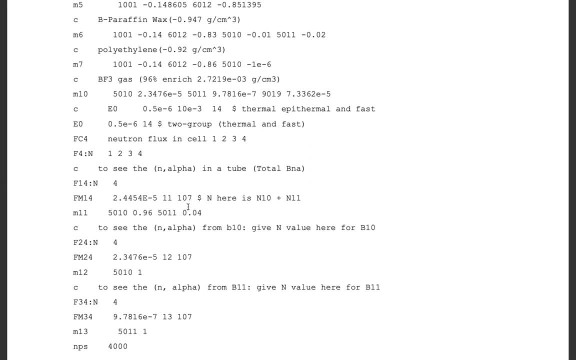 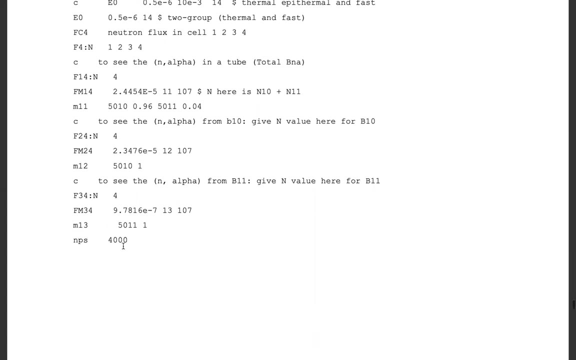 is boron and 107 is the microscopic cross-section for an alpha reaction. so then i did this again for b10 and b11 separately. i ran this simulation for 4 000 particles, which is very small when you're doing a paper or or your phd thesis. i remember my student took 400 000, so 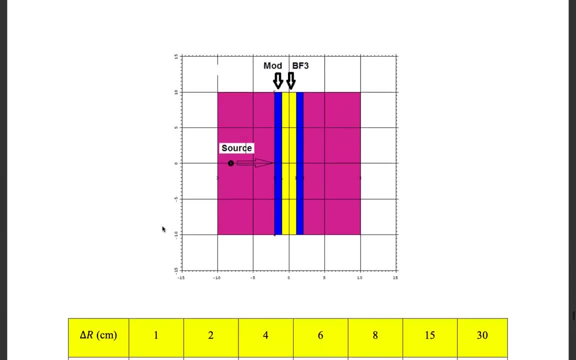 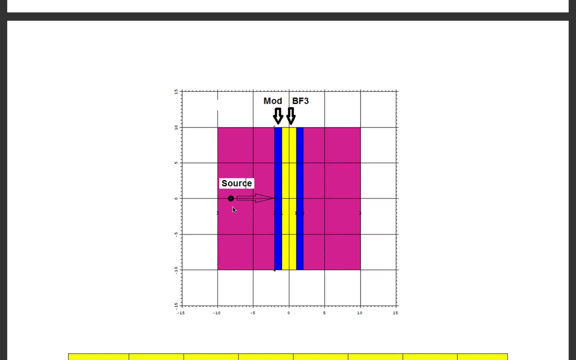 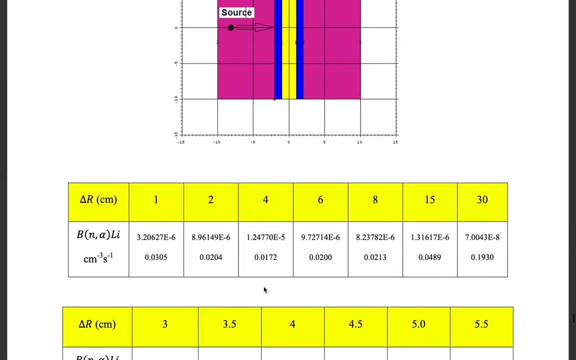 carry out a big, proper simulation. now these are the results which i'm going to show you. this is one tube, so yellow is the gas and the blue is the moderator and purple is some other medium in which the source is placed and fired. okay, that's surface one, surface two, and try to make the input files yourself. 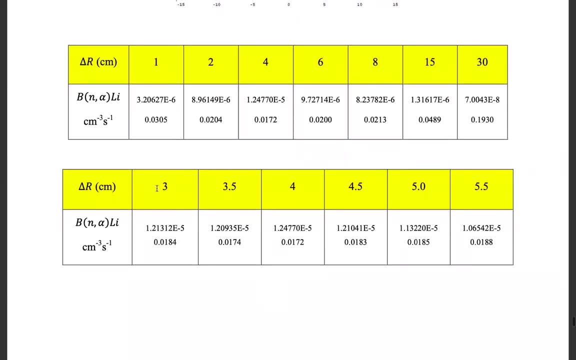 if you want me to send you, you can email me and i'll send you. okay, now, in this study you can see that we varied the moderator thickness in front of between the source and the bf3 tube and we did a count on the nl4 reaction. so can you see, 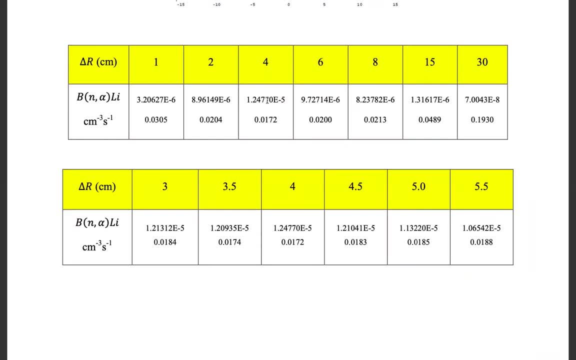 that when it's going up from one to two to four centimeter, our source is not. it goes up but then it starts going down. so somewhere between four and six centimeters thick. I think this is, Rex. we've got the optimal. so what we did over here was that we looked at this region three to five, point five a little. 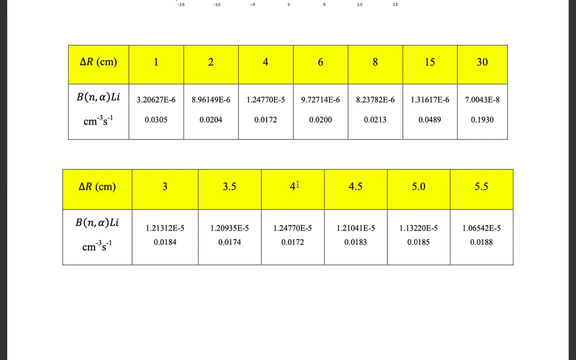 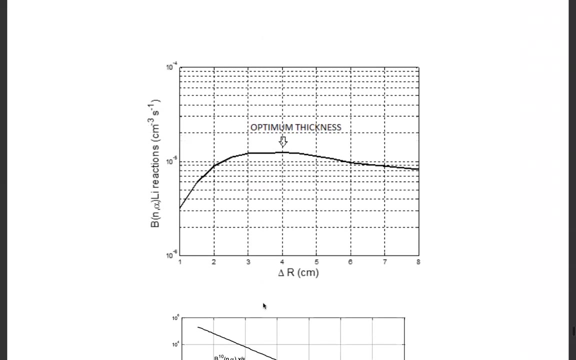 bit more carefully and you see that somewhere over here is the maximum. so so why is it so important to get the optimal moderator thickness? because you're going to take something out of the field and you want the best possible optimized design. so when you plug these numbers over here, you see that as a 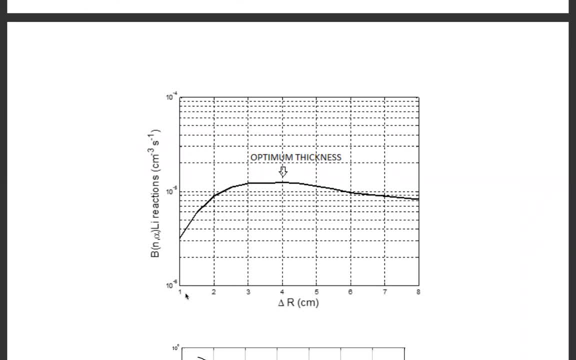 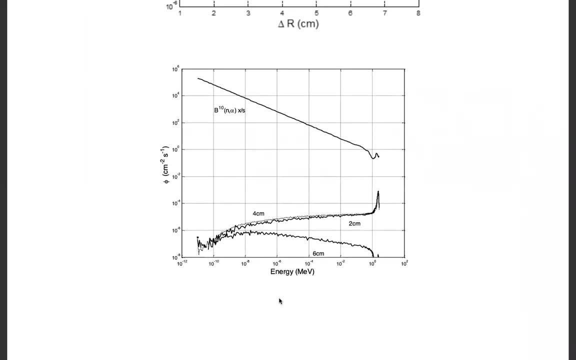 function of the thickness of moderator delta R in centimeters. so the B and alpha reaction rate goes up, up, up, stabilizes, saturates and that starts coming down. so here's the optimal thickness, about four centimeter. now this depends on the, on the material of the moderator. 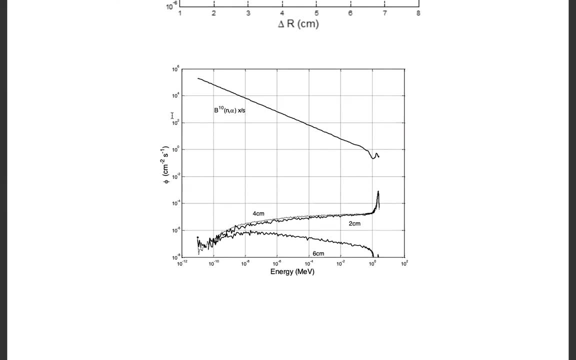 so what we did was that here you see energy and flux plotted now here I think we have more than a hundred evaluations of flux, so made about a hundred or more energy bins big input file. so we saw what the spectrum looks like for two centimeters. see then for four centimeter also. it's good, but if you exceed four, 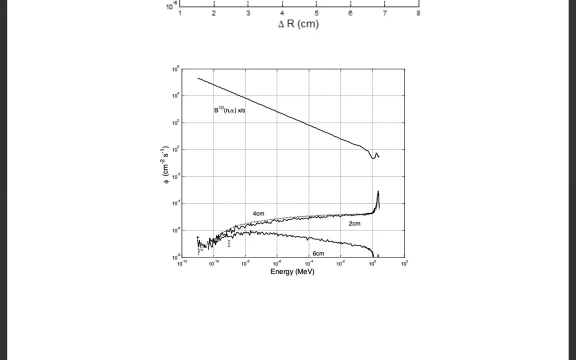 centimeters and look at the spectrum it reduces in this end, as well as in data and the B and alpha cross-section. just to show you, on the same figure in in ten- I sort of five be ten- you can see that it goes up on the log scale. so so, yes, we. 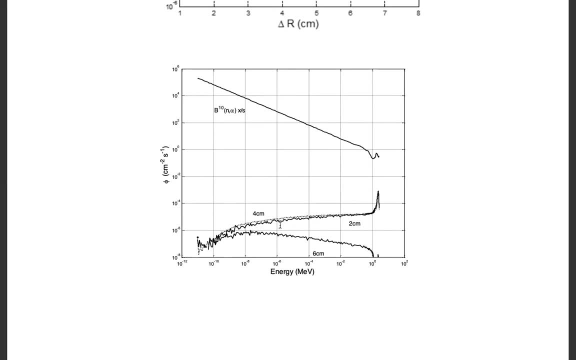 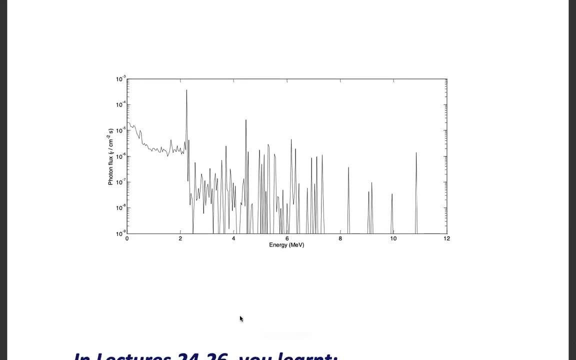 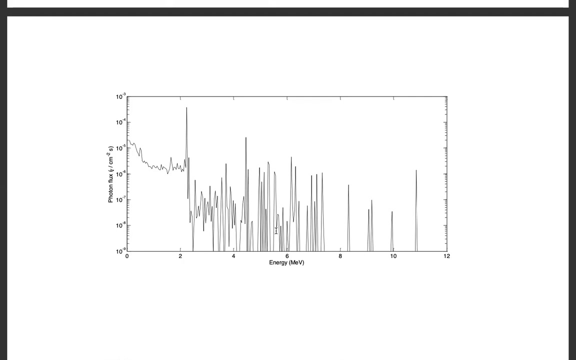 do want thermal neutrons. so this shows you that there's an optimum close to about four centimeter. so this is the study that you need to carry. this is the signal that we get from our portable detector, and now this signal has gone out so many, so many pulses. and can you see that? this is two point two, two MEV. so 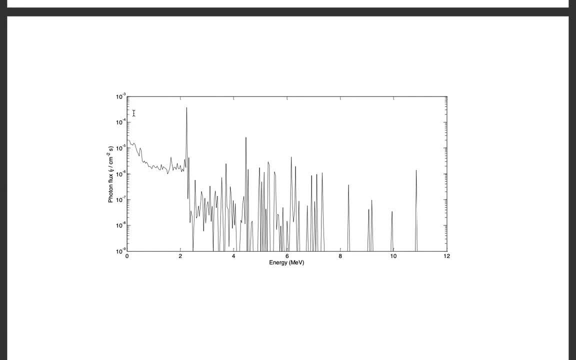 this is the nice hydrogen peak we've got about. so this is ten thousand twenty thousand thirty thousand- sorry, this is ten to the minus four neutrons and photons per centimeter square per second. so you've got to multiply this by the californium source strength, which is about ten to the seven. 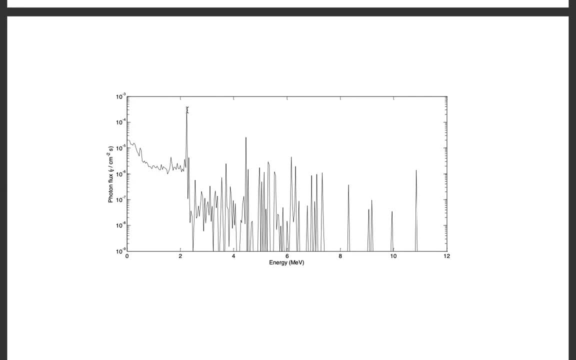 so when you multiply this by ten to the seven, that we took out ten to the eight, so you get about twenty thousand pounds over here. so you get about twenty thousand pounds. and then of course you've got to do a study that what is the soil in your area? is it calcium carbonate, limestone, is it sand? what is? 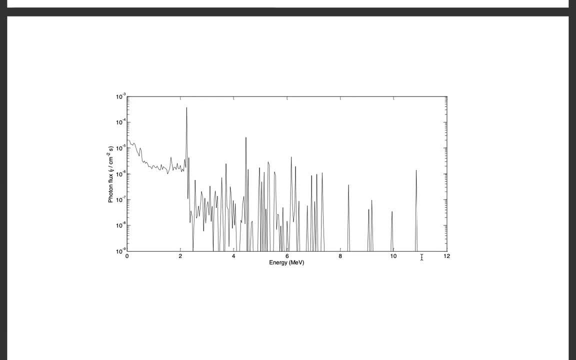 it. and so this is the nitrogen peak that you see, the ten point eight MEV. these are the other peaks, and you've got to see tables of the various peaks that you get. so from the relative intensity of this to this, you identify whether you have an explosive or not, and then you work out the chemical. 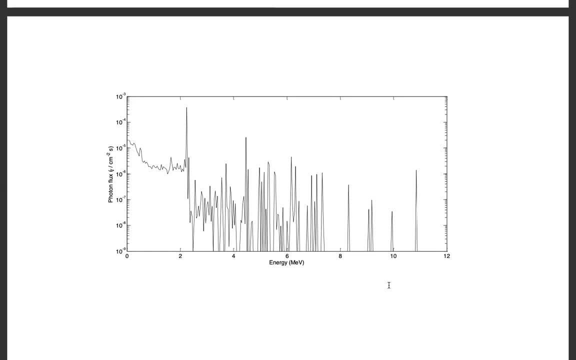 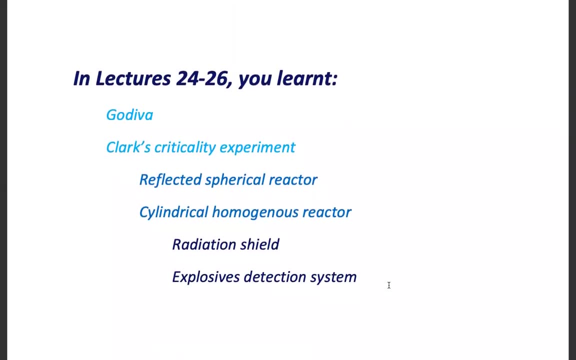 formula of this unknown sample and from that we did all the simulations and we found that, yes, you can detect explosives, and and these things are being developed and in the next few years you'll find these kind of explosives which are freely available and used at airports and dry ports and when cars are entering. 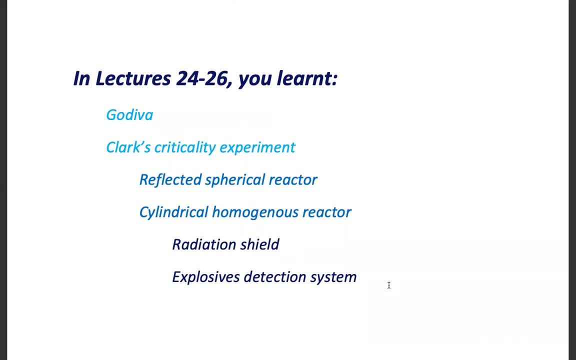 cities leaving, you know. so for the safety and security systems and for humanitarian demining, which is so important. okay, so in these lectures you learnt applications of Monte Carlo simulations. these are very, very strongly recommended to to nuclear engineers, and you see, the theory that you study in your classroom is for a purpose and 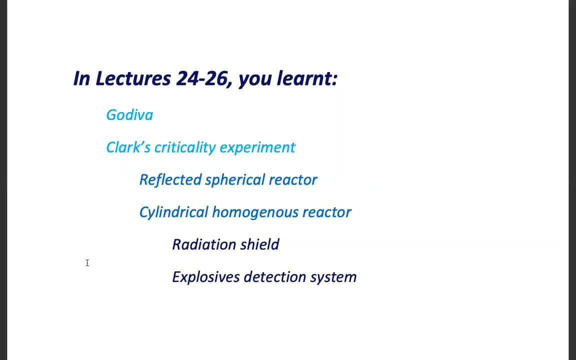 that purpose is to design nuclear systems, because before you go and do anything practical, you must simulate. because nuclear is a field where safety, just like industry, just like any engineering thing, safety is the most important thing. after safety comes economics and functionality. so nothing, nothing, nothing is more important than 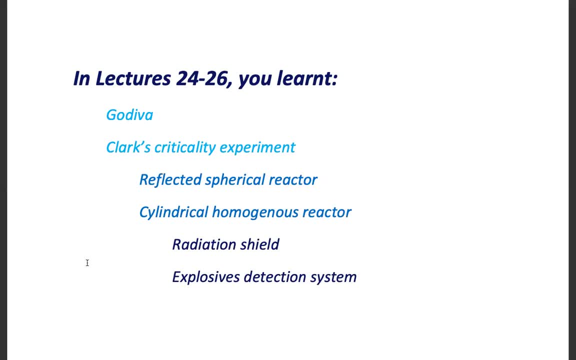 safety and if you read about industrial accidents you'll see. read about Chernobyl, read about the Bhopal Union carbide accident and there are so many industrial bad things that happen where people lose their lives. so as engineers, our foremost consideration is safety. so in the last few years we have seen a lot of 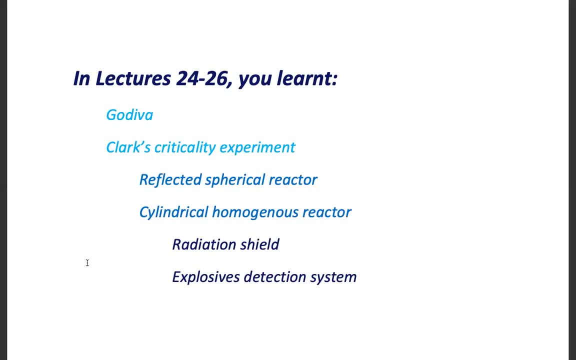 new changes and there are many new approaches in this course and the Feel you, if you are interested in in this course, any forward to my objective. as somebody who's worked 35 years, after which I had a small one year, my first experience was an Exxon chemicals at the fertilizer plot which operates at 3000. 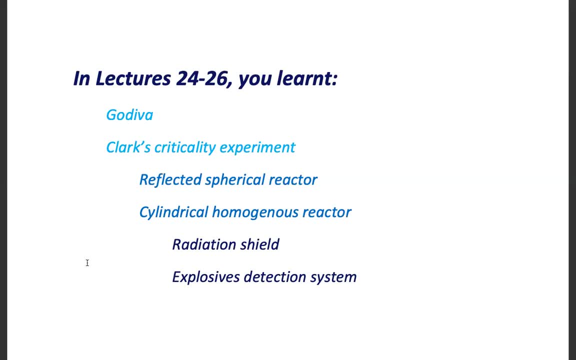 PSI. so you know, chemical industrial safety is so important, nuclear safety so important. so that is why, in these three or four lectures I took you through practical applications, which often in every school is a vehicle which you take to the undergraduate studies. we are not taught, and i certainly wasn't, and so i learned, because in 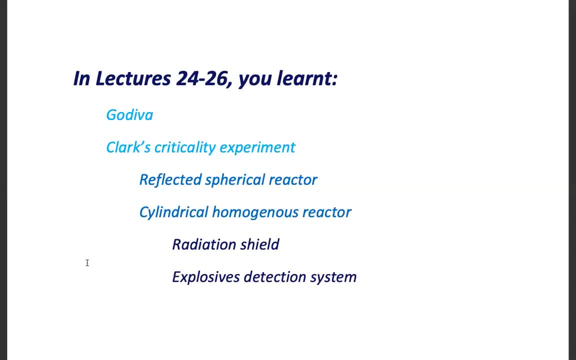 those days we didn't have so many computer codes, we didn't have systems, we didn't have the internet, we didn't have laptops, so we were a bit slow. we had to read books and you know our education was very different. so your education, especially in the lectures, and these lectures which i'm 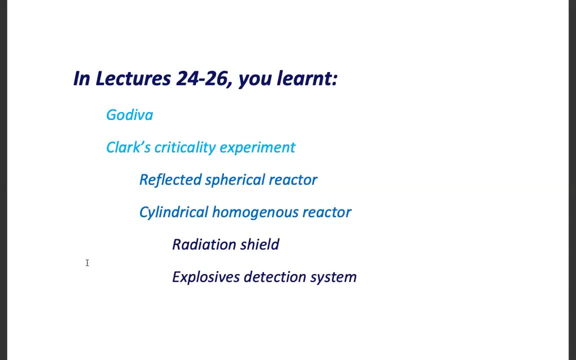 uploading on youtube. i think that i'm giving all that i have learned and- and really this is wealth- of tying up your theory with applications, and if you have seen these things with your eyes and you touch them, then you understand which equation applies over here. and, believe me, when you're in, 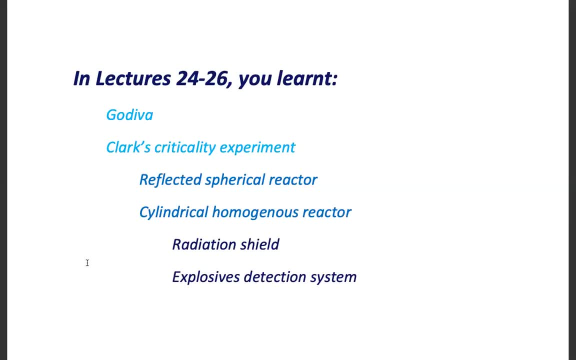 a work environment, you don't have time to read books, you have time to do things because industry allows you to do things and you have to be so fast that it's your reflexes which are important. okay, so i hope you've learned godiva, you've learned clark's criticality experiment, you've 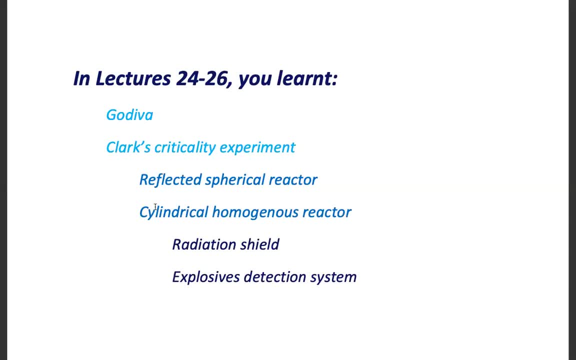 learned: reflected spherical reactors, cylindrical homogenous reactor, radiation shield, explosive detection system. i am now confident that you can go and tackle any big problem and you will see that you understand things and you understand the physics of it and you can solve it. you understand the mathematics of it, you understand the science of it, you understand the.